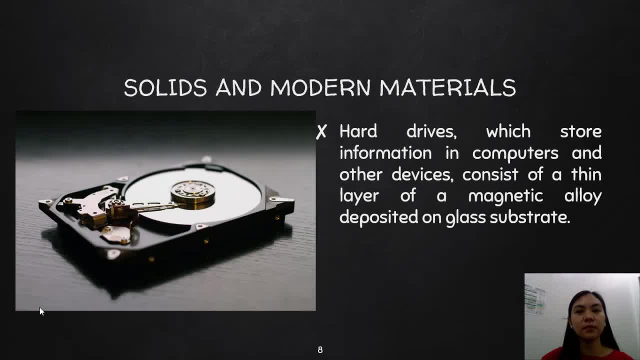 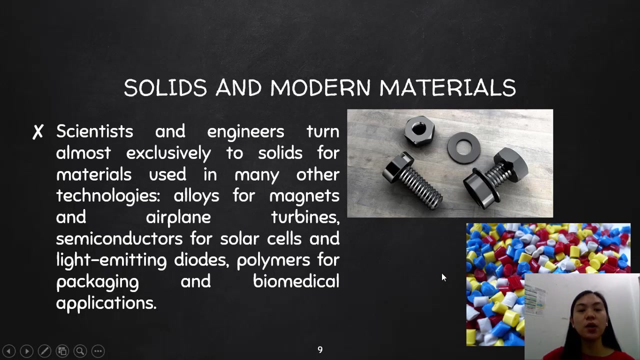 insulators like hafnium oxides, Your hard drives which store information from your computer and other devices. they actually consist of a very thin layer of magnetic alloys deposited in your glass substrates. Your scientists and your engineers almost turn exclusively to solids for materials used. 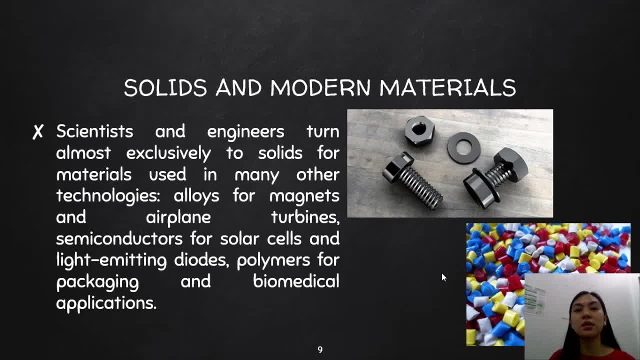 in many other technologies. So it's very obvious that, for example, the current device that you're using to watch this video, they are actually made out of solids And, of course, all of those materials that you're holding right now are possible because of the solids that we could harness from nature and turn. 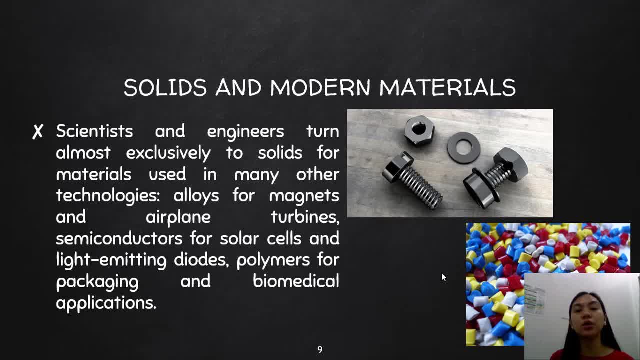 them into modern materials that we could use in order to help us in our daily lives. So it says here: alloys for magnets and airplane turbines, semiconductors for solar cells and light-emitting diodes, polymers for your packaging and biomedical applications. 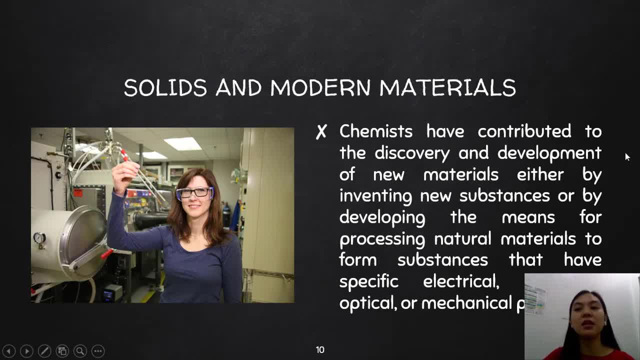 So chemists have contributed to the discovery and development of new materials, either by inventing new substances or by developing the means for processing natural materials to form substances that have very specific electrical, magnetic, optical or mechanical properties. Of course, when we want to use something, for example, we want, for example, 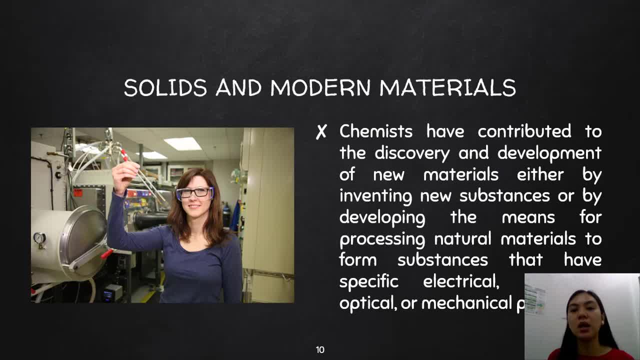 your gadgets, your integrated circuits inside your gadgets, There are specific solids that we need to use in order for us to meet the criteria that is needed. So your solids: they have different properties, which we will be covering later on, And whenever you're chemists. 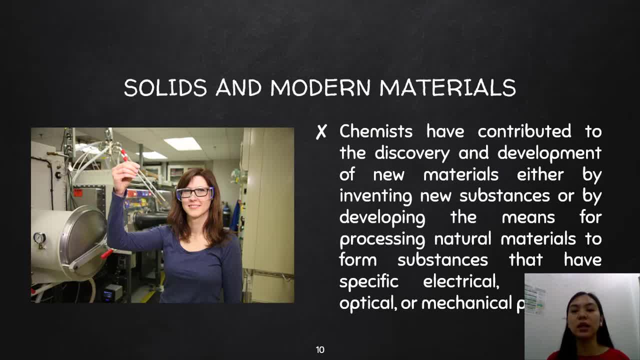 scientists and engineers want to use a certain solid, they have to make sure that it actually conforms to the needed criteria, like your electrical property, optical property, magnetic, mechanical and even sometimes chemical properties. Slide ace, Slide actor, Slide mister, Slideишь. 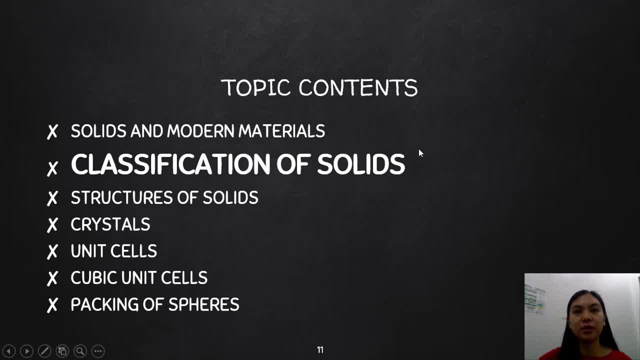 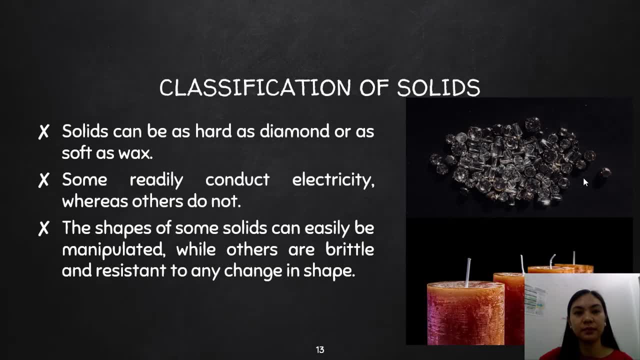 Slide, Slide, Slide, Slide, Slide. the second topic for this particular um content, so the classification of your solids. so, uh, our solids uh is there, or rather are very different from each other, as you can see here in the first statement. they can be as hard as a diamond or even as soft as wax, some readily. 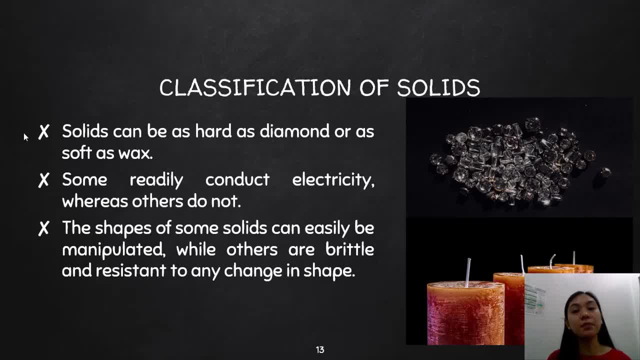 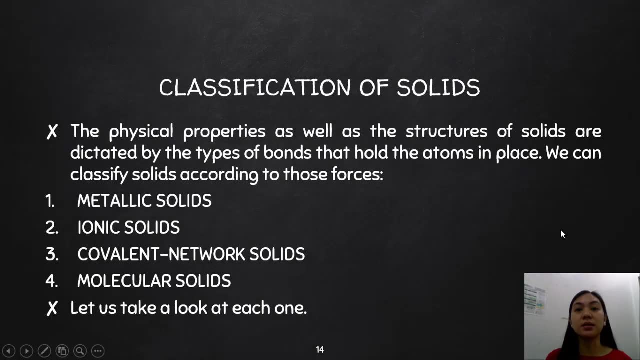 conduct electricity, while others do not. some can. some can be manipulated into the shapes that you want, while others are very resistant to any change in shape. the physical properties, as well as the structures of your solids are dictated by the types of bonds that hold the atoms in place. 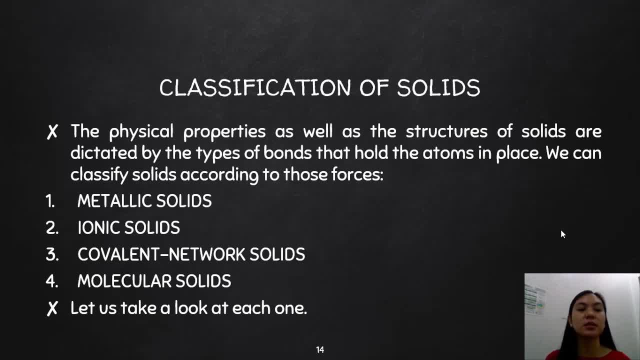 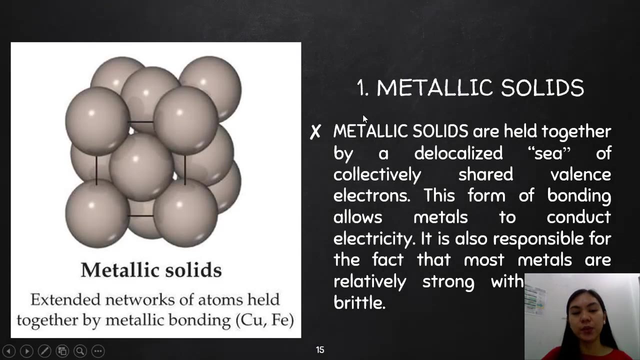 and we can classify your solids according to those forces. so you have four classification of your solids: mainly your metallic solids, ionic solids, your covalent network solids and, of course, your molecular solids. now let us take a quick look at each one of them. so your metallic solids: when we say metallic solids, they are held. 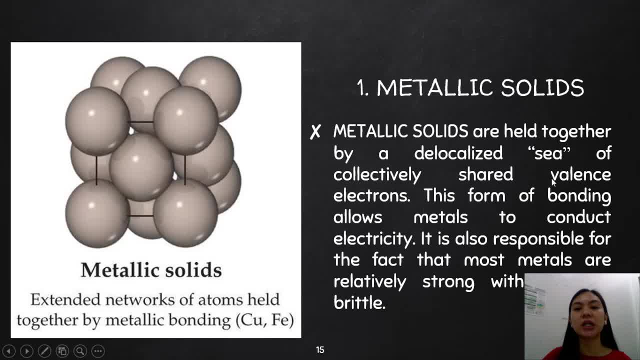 together by a delocalized sea of collectively shared valence electrons. this form of bonding allows metals to conduct electricity it is. it is also responsible for the fact that most metals are relatively strong without being brittle. so your metal metals are very specific kinds of solid because they actually have like um. of course you already know that. 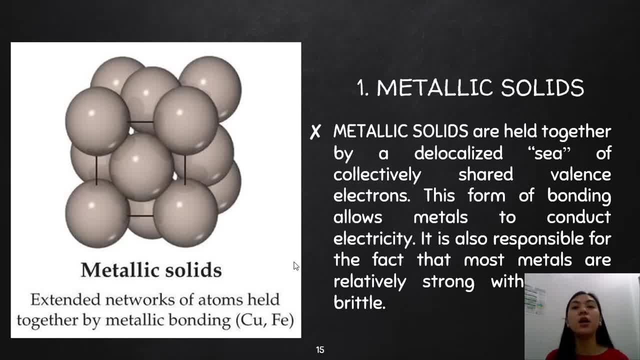 your atoms, or rather your atoms, is composed of your nucleus and your um electrons. now you can also see that the electrons are being shared with each other. so in metallic solids the electrons from atom to atom are being shared, meaning they can travel from one nucleus to another. that's why they call it your, the localized c, because it is very much. 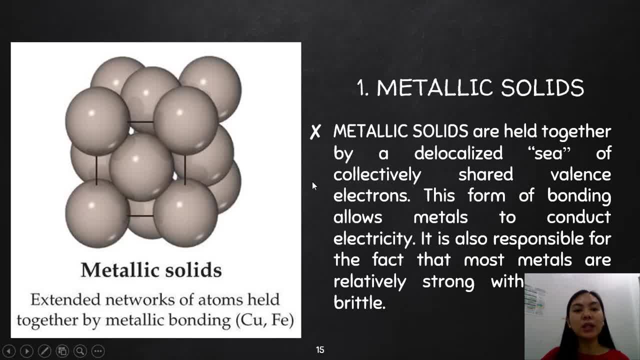 c of collectively shared electrons. now, because your electrons can travel from one nucleus to another like free-flowing electrons. that's actually the reason why you can see the difference in the number of electrons in the metal and the number of electrons. that's why we turn exclusively to metals when we uh for your copper wires, for example, because 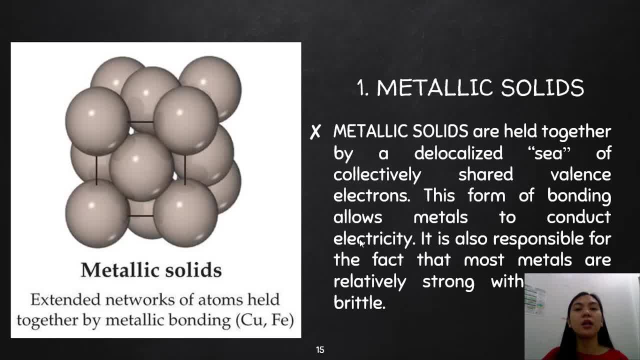 your electrons can flow and for your gadgets. we're actually using metals because of this particular property, wherein you have a sea of electrons. but we'll talk about metals more in the upcoming video, since we have a very specific topic for metal. so let's talk about metals now. 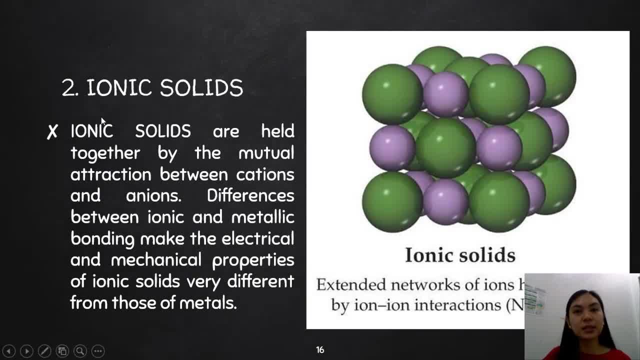 first of all, let's talk about this. so the next type of solid is known as your ionic solids, when we say ionic solids from the name itself. from the name itself. it is composed of ions and these are held together by the mutual attraction between your cations and anions. differences between 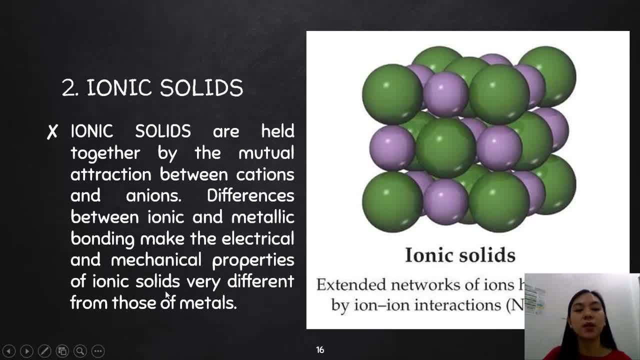 ionic and metallic bonding make the electrical and mechanical properties of ionic solids very materials. so when we say ionic solids, this are made up of one metal and a non-metal. so the bonds are you have um. when you say ionic, they say the electron one one. 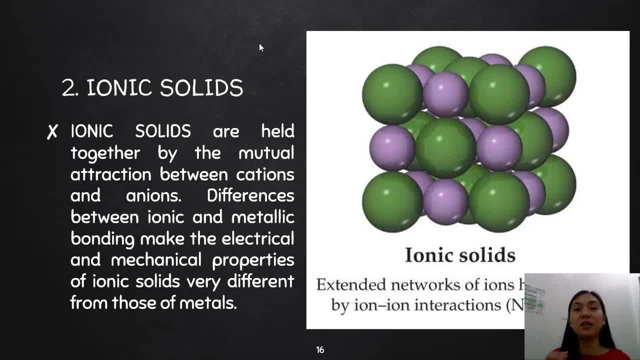 element will be sharing, right, we'll be giving up, rather, the electron. so we'll be. we'll be giving up the electron to the other element. so, for example, you have your nacl here, your na is a has a charge of positive one and your chlorine has a charge of negative one. so ibig sabihin: po si sodium ion dito. 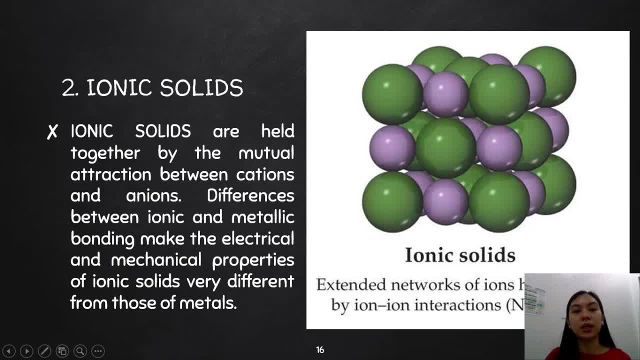 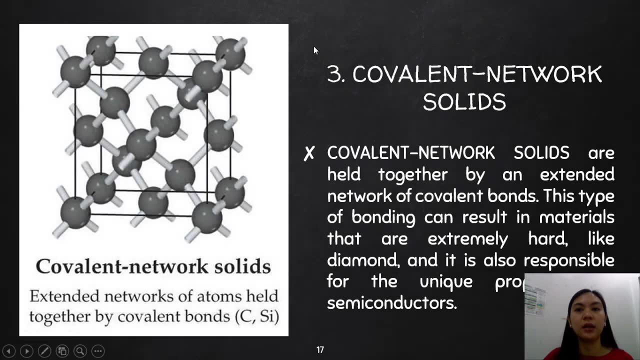 i give up niya, yung electron nya papunta kay chlorine, para po they could reach your stability. so it's giving up of electrons and yung pag give up ng electrons na yon, yun po yung mag may make ng bond nilang dalawa and you have the third one, you have your covalent network solids. 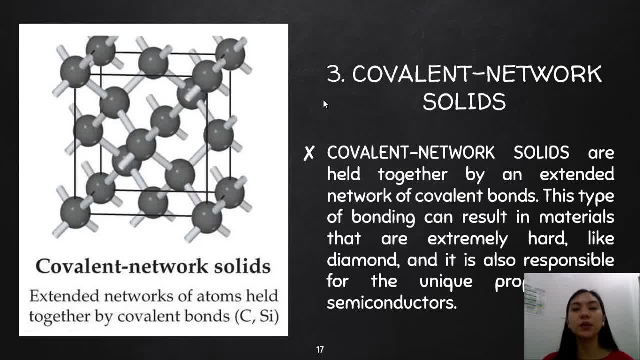 when we say covalent network solids, they are held together by an extended network of covalent bonds. now, when we say covalent bonds, ibig sabihin po dito yung electrons. sinishare po ng dalawang element diba. kung sa ionic bond po yung electron is, i give up. however, dito sa covalent bond, magsha share. 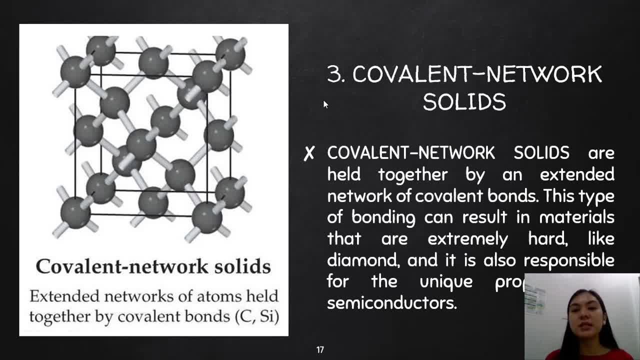 sila doon sa electron. so it says here: this type of bonding can result in materials that are extremely hard like diamond, and it is also responsible for the unique properties of your semiconductors, your covalent network solids. um ito po yung mga strong solids kasinga. 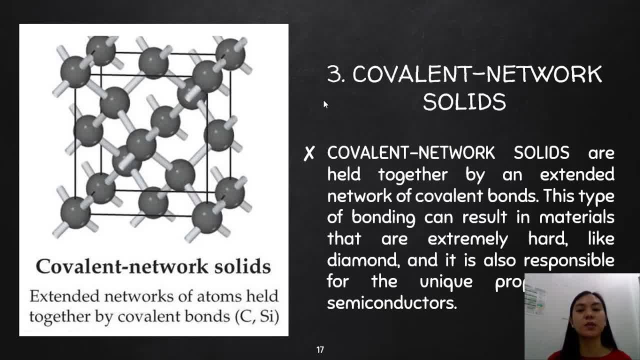 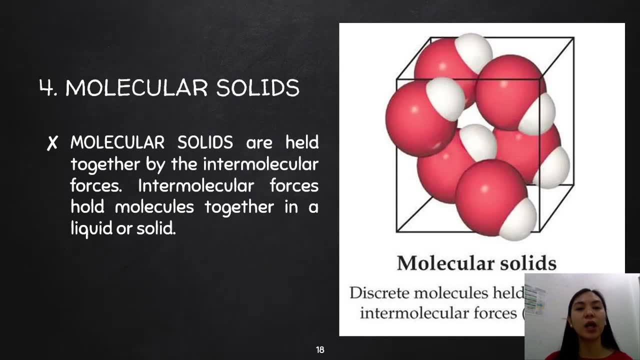 as Because the electron is being shared, so the force is stronger compared to your ionic solids. So that's it. And of course, the last type are your molecular solids. When we say molecular solids, on the other hand, these are held together by your intermolecular solids. 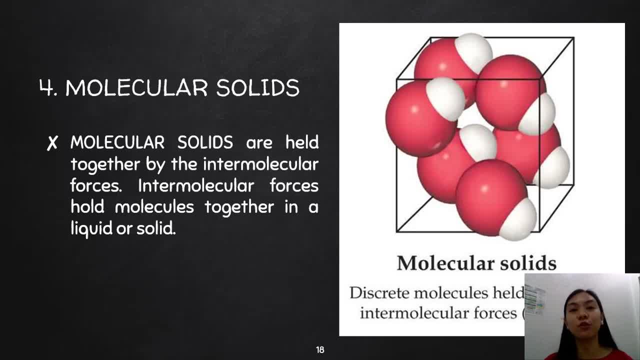 When we say intermolecular- sorry, intermolecular forces rather- And when we say intermolecular forces, this is the type of force that holds molecules together in a liquid or solid. An example of this is your water. So dito water. 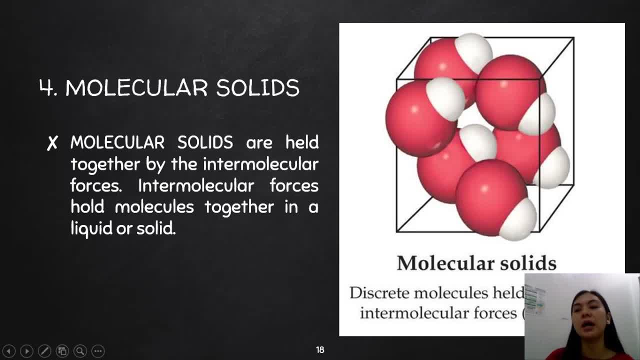 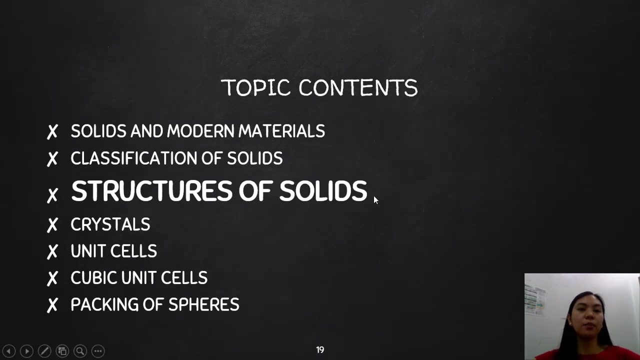 Diba Yung water nyo kasi nage-exist siya with an oxygen and two hydrogen atoms, So they are being held together by your intermolecular solids. It exists as a molecule. So let's go to the third topic of this content. 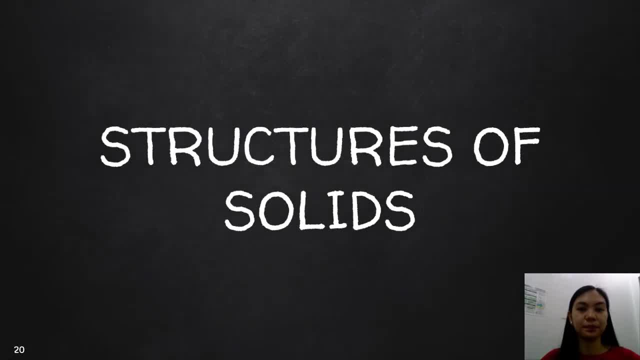 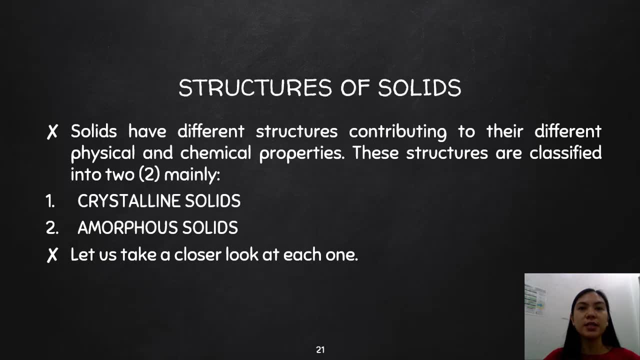 You have the structures of solids. It says here. solids have different structures contributing to their different physical and chemical properties, And these structures are classified into two mainly: your crystalline solids And your amorphous solids. excuse me, Let us take a closer look at each one of them. 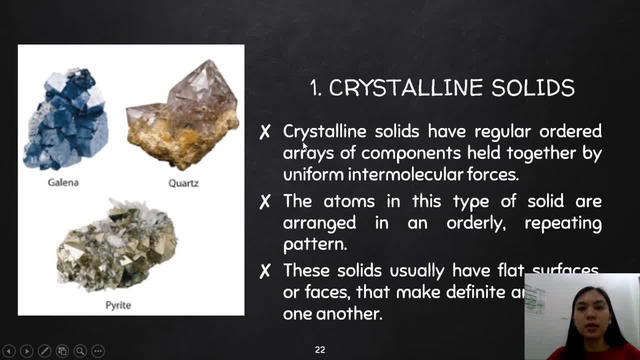 When we say crystalline solids, these are solids having regular, ordered arrays of components held together by uniform intermolecular forces. Now, the atoms in this type of solid are arranged in an orderly, repeating pattern. These solids usually have flat surfaces or faces that make definite angles with one another. 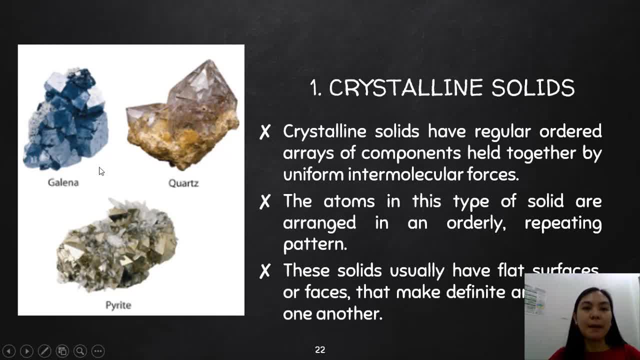 So, as you can see, you have here examples of your crystalline solids, You have your galena And if you take a look at the picture, parang siyang tumutubo siya, in such a way na parang you have little cubes. 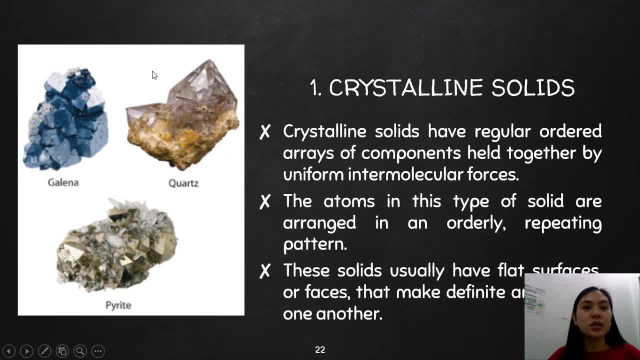 Diba Ganyan, And you also have your quartz. Tapos, yung quartz naman parang tumutubo siya, in a way na parang papir Pyramid yung kanyang structure. And you also have your pyrite. 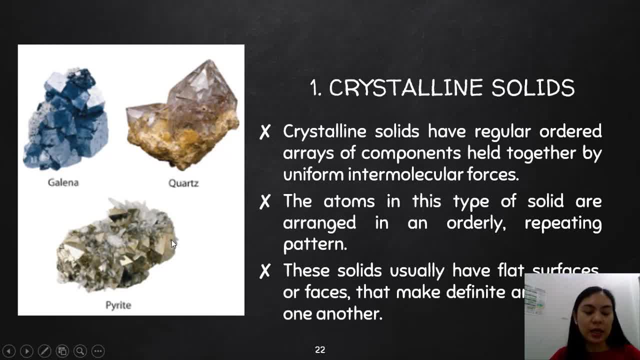 Medyo magulo siya, but there's actually a certain pattern to this. Kaya mong bigyan ng pattern to your pyrite, So parang siyang much more like the structure of your galena as well. Kung baga parang may mga nagpoform na cubic shapes here. 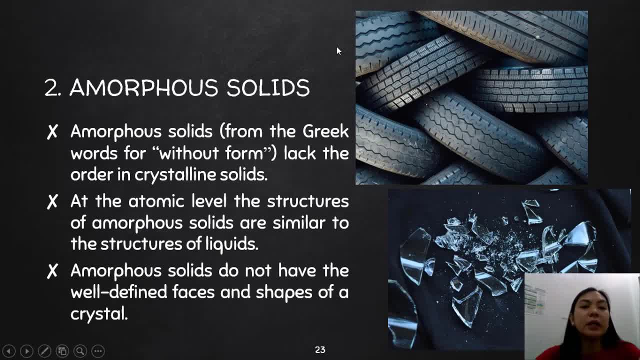 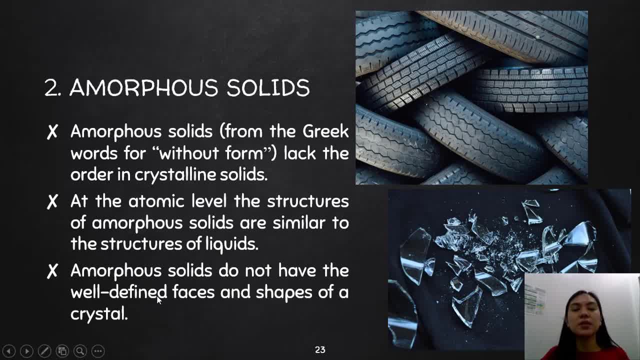 Amorphous solids do not have well-defined faces and shapes of a crystal. Amorphous solids do not have well-defined faces and shapes of a crystal. So when it comes to crystalline solids, we have very definite patterns. For amorphous solids, they do not have any patterns. 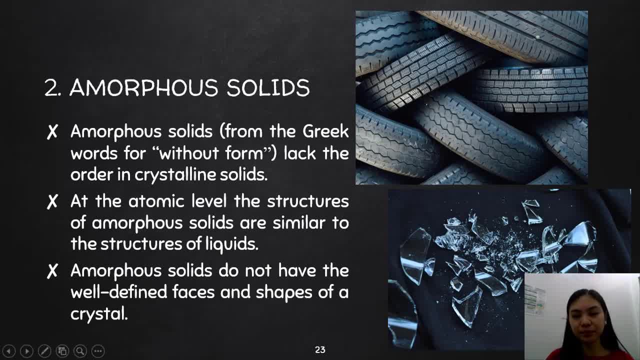 An example of this is your glass. Glass is a type of an amorphous solid. That's why glass, when it falls or breaks, you will not see the pattern of the pieces that broke, Just like in this particular picture. they vary in sizes and in shapes whenever they break. 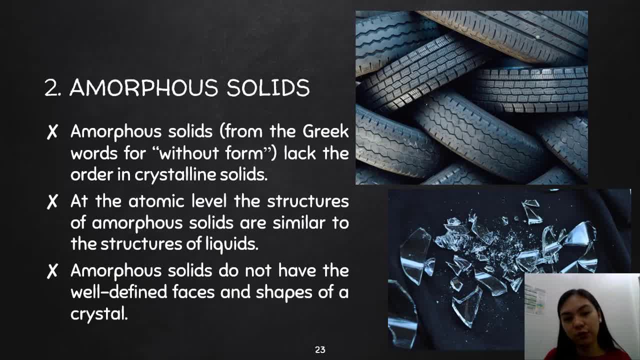 Because it's an amorphous solid. they do not have any form. Another example is your rubber. Rubber is very soft So it really doesn't break. It really doesn't have any molecular or atomic form. That we will be discussing later on. 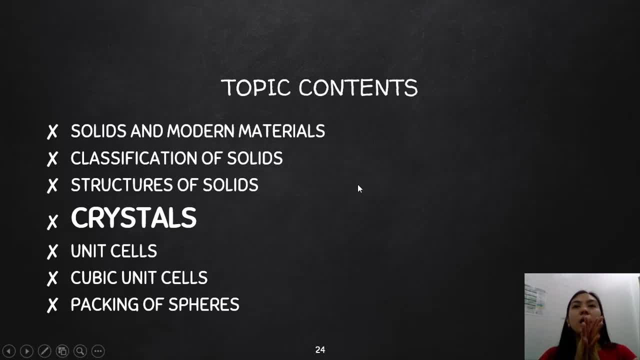 So, among the two structures of solids, we will mainly focus on your crystalline solids, Or your crystalline solids are commonly denoted as your crystals. We will focus on those because they have shapes and patterns. In an amorphous solid, there is no shape or pattern. 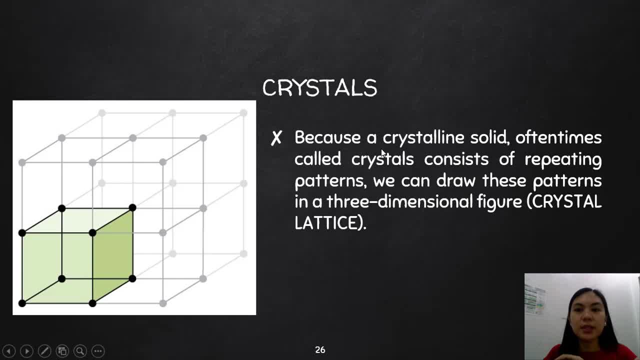 So it says here: Because a crystalline solid, oftentimes called your crystals, consists of repeating patterns, we can draw these patterns in a three-dimensional figure called your crystal lattice. So structurally we can draw the structure of a crystalline solid. 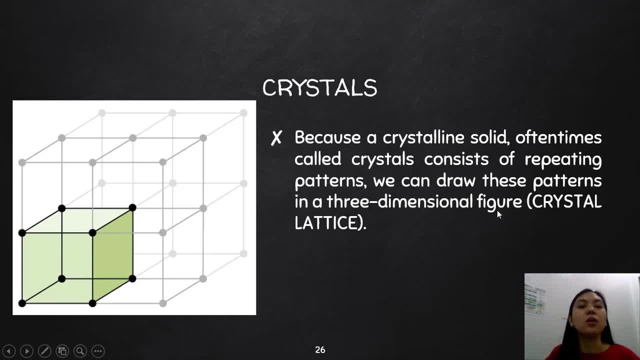 And that three-dimensional figure which represents the solid is called your crystal lattice. So this is what it looks like. Let's imagine that these are either ion or atom or molecule, And of course the ions will stick together. So we will draw it this way so that we can imagine how they actually look like in a molecular 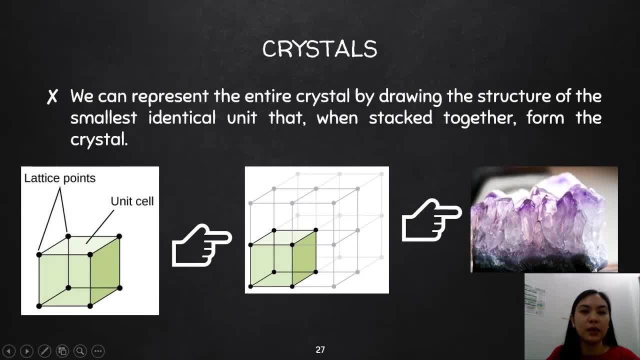 So, as you can see here, we can represent the entire crystal by drawing the structure of the smallest identical unit that, when stacked together, form the crystal, by form the crystal. So, for example, this is the smallest unit that can represent the totality of the crystalline solid. 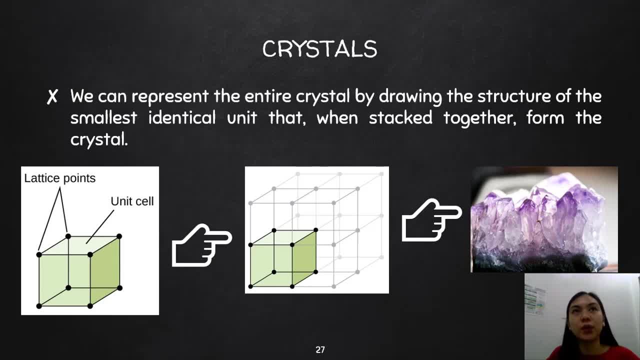 In other words, If we try to imagine right, For example, your sugar, your sugar granules, For example, one granule is still a representation of the whole bag of sugar. For example, you have one kilo of sugar, right? 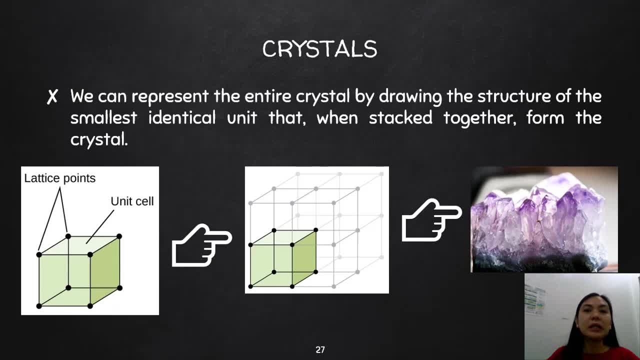 The smallest particle is still sugar. So that is how we can imagine when we talk about crystals. So you have what we call your unit cell. Then, when your unit cell is stacked together, right, You will have your crystal lattice, And that particular crystal lattice will represent the totality of the crystal. 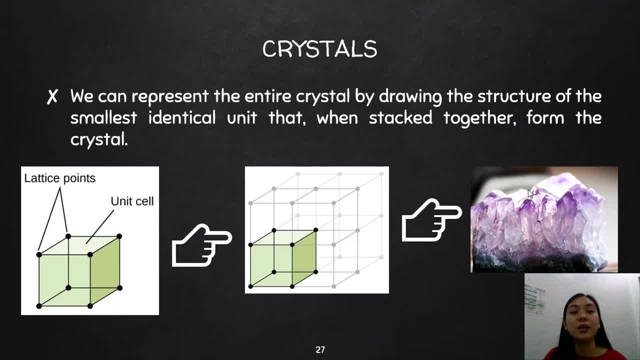 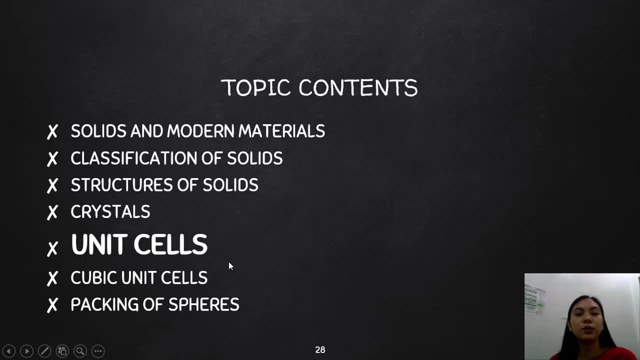 So that is how we can do representation for us to understand your crystals in the smallest possible unit. Okay, Alright, So now that we already have that, let's go now to what we call your unit cells. So what is a unit cell? 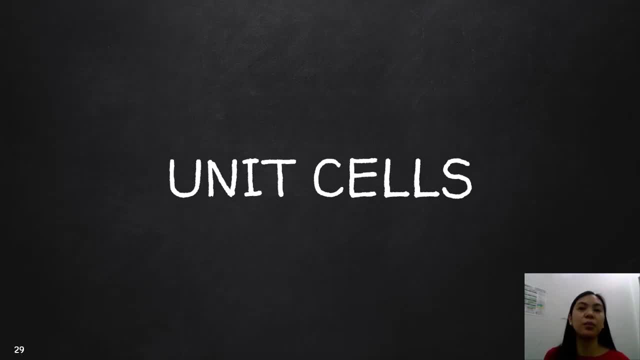 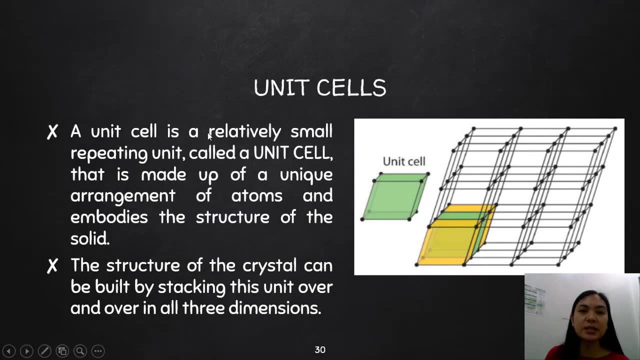 You already mentioned it earlier, But let's dig deeper on what it really means. So it says here: A unit cell is a relatively small. I'm wrong here, So this is a grammatical error. So a unit cell is a relatively small. 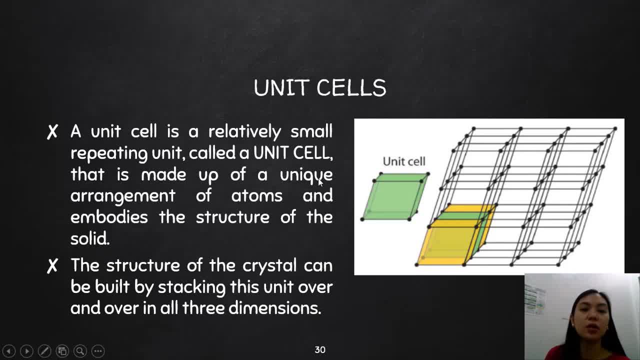 that is made up of a unique arrangement of atoms and embodies the structure of the solid. So the structure of the crystal can be built by stacking this unit over and over in all three dimensions. So, as you can see here in the figure, that is our unit cell. 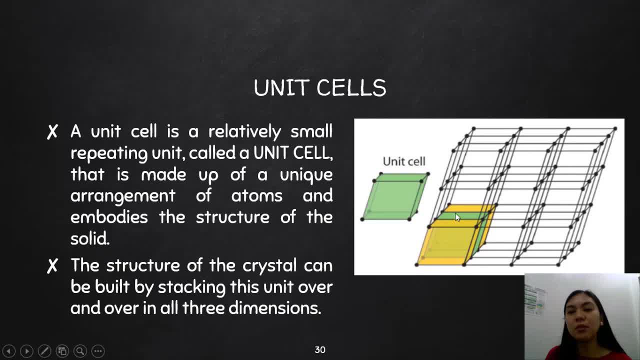 And then this is another unit cell. So when you stack the unit cell together you could actually embody the whole structure of your crystalline solid. So just imagine that in a bag or a kilo of sugar the smallest granule is the unit cell. 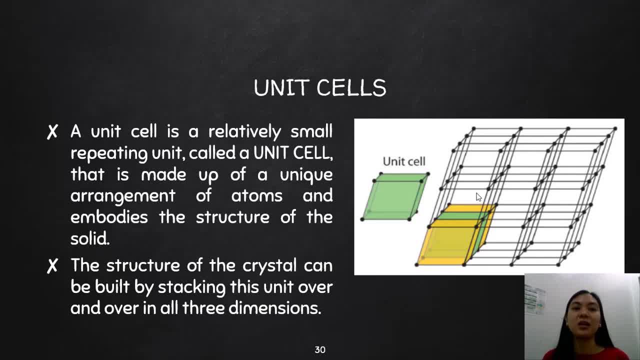 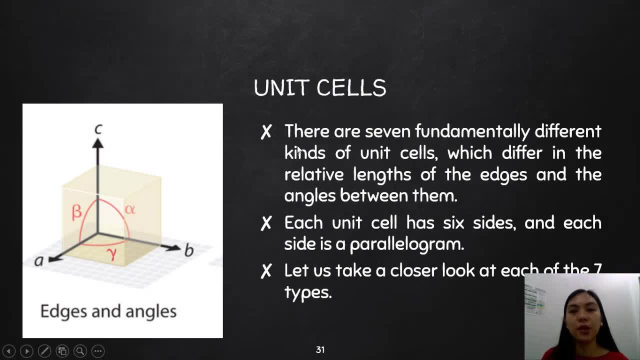 Because it will still be sugar, it's just that it is in the smallest form, Something like that. So it says here There are seven fundamentally different kinds of unit cell, which differ in the relative lengths of the edges and the angles between them. 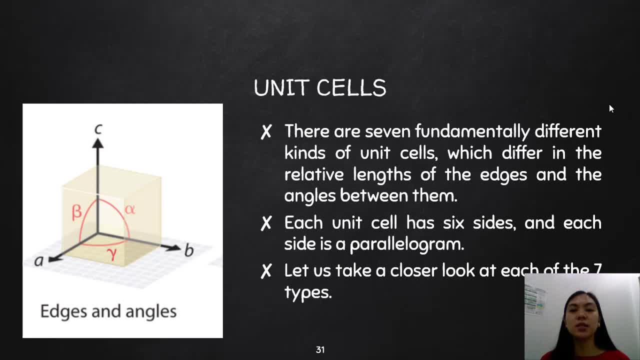 Each unit cell has six sides and each side is a parallelogram. Let us take a closer look at each of the seven types. So if you imagine the unit cell, of course it's three-dimensional right. So we will represent the seven types of unit cell. 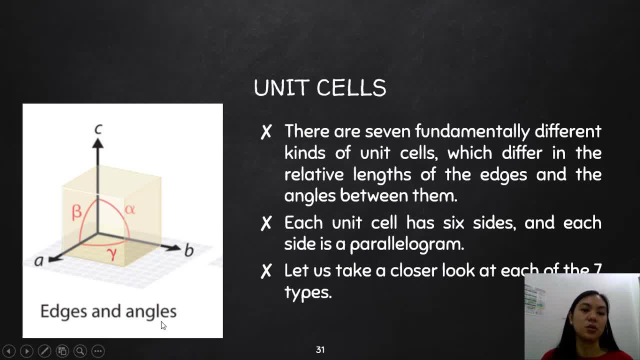 following the edges and the angles. So if you take a look at the figure here, you have your y-axis represented by your letter C, your z-axis represented by your A and your x-axis represented by your B. So the sides are represented by your edges A, B and C. 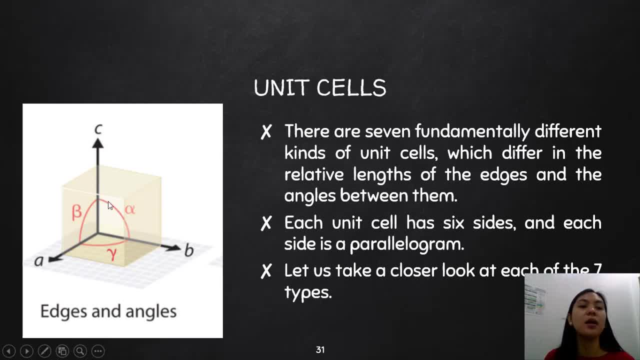 and then the angle that each side made with each other is represented by your Greek letters alpha, beta and gamma. So it looks like this: So you have your sides and then you have your angles- alpha, beta, and then your gamma. 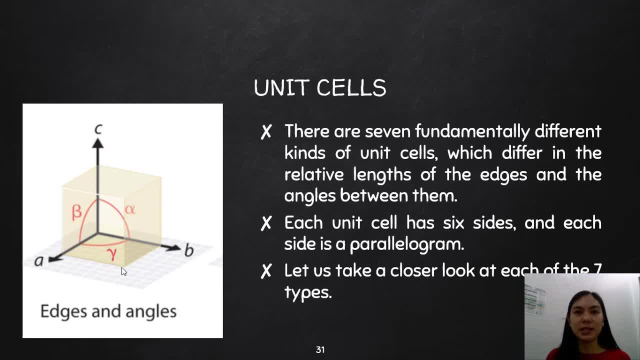 So this is how we will imagine each unit cell, because unit cells for different types of solids are different, Because they are not all cubic or they are not all of the same structure. So we will dig deep on how these unit cells actually look like. 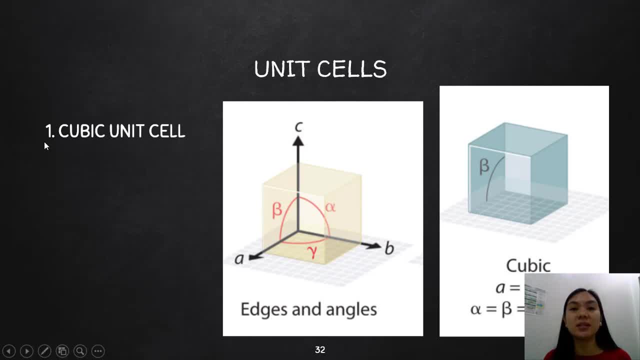 So let's have your first unit cell. We call this your cubic unit cell. It's the simplest among all of the unit cells, So it seems easy because it's simply a cube. So it means, if it's a cube, right. 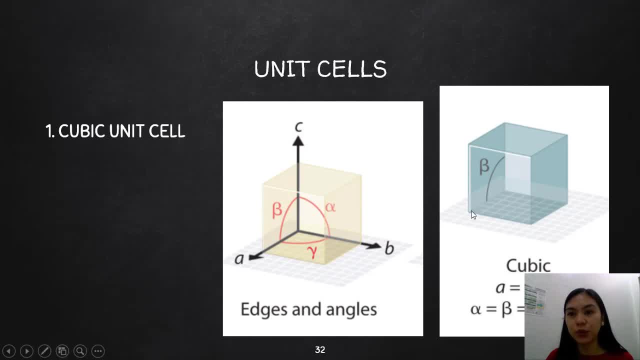 Your line A is equal to your line B and is equal to your line C Because they have the same size of edges or the length of the edges And, of course, since it's a cube, you all know that the angles alpha, beta and your gamma. 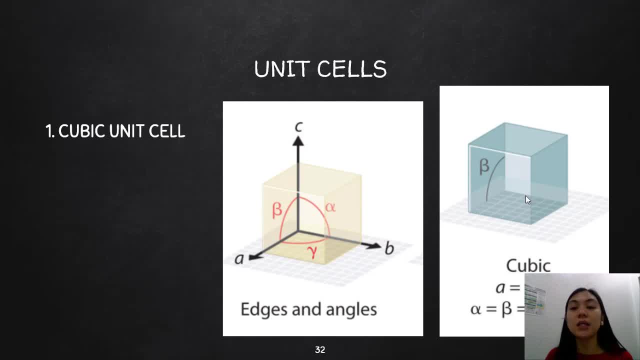 are actually equal to 90 degrees Because the sides are perpendicular to each other. So that is one type of unit cell. It's just like a cube, So it's a cubic unit cell. Imagine that the granule of sugar is a perfect cube. 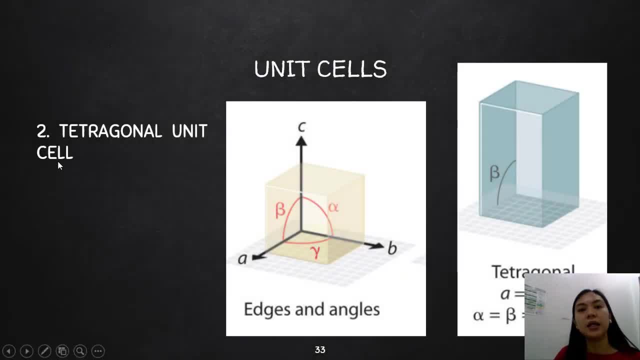 It's just like that And you have the second type of your unit cell, which we call your tetragonal unit cell. Now, when we say tetragonal unit cell, as you can see right, Angles A or rather sorry. 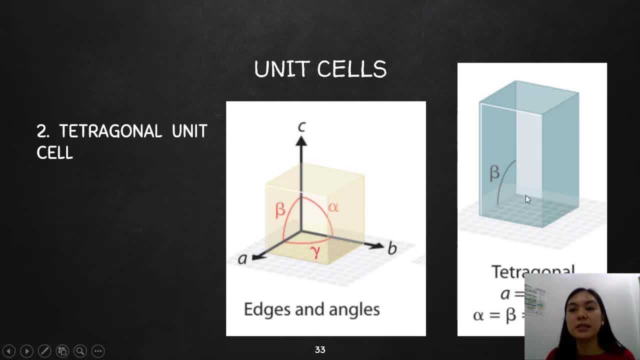 side A is equal to the length of side B, So you have a square there. So side A is equal to side B. However, side A and side B is not equal to your side C. So, as you can see here in the figure, 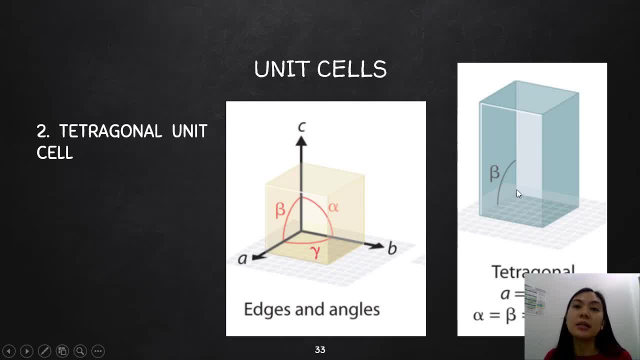 the side C can be longer, but the side C can also be smaller, So it's not the same size, And although the angles that they make with each other are 90 degrees, which means that they are perpendicular to each other, So the side C is the only difference. 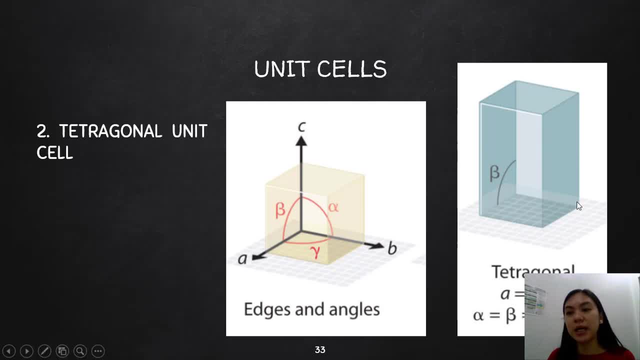 Okay, So your side A is equal to your side B. However, they are not equal to your side C, Although all of the angles- alpha, beta and gamma- is equal to 90 degrees. So that is the second type of unit cell. 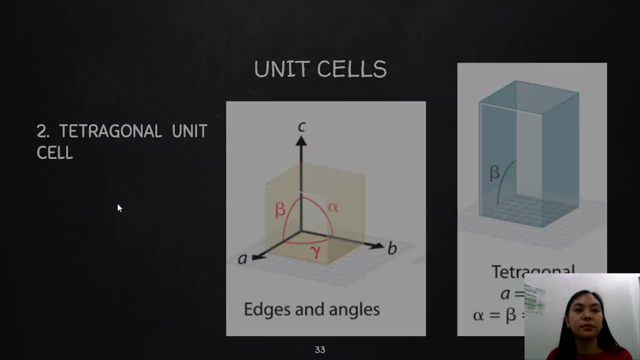 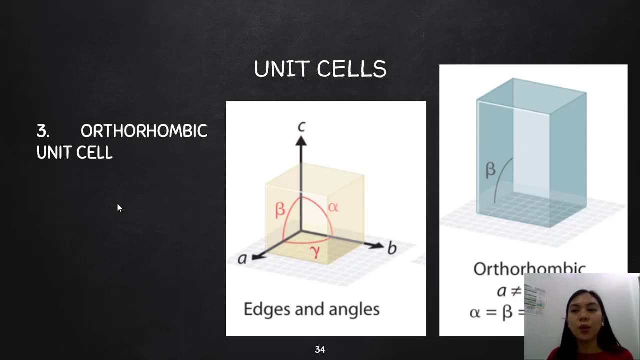 Your tetragonal unit cell. And then we have the third one, Your orthorhombic unit cell. Now, when we say orthorhombic unit cell, you can see here, these are the edges and these are the angles. 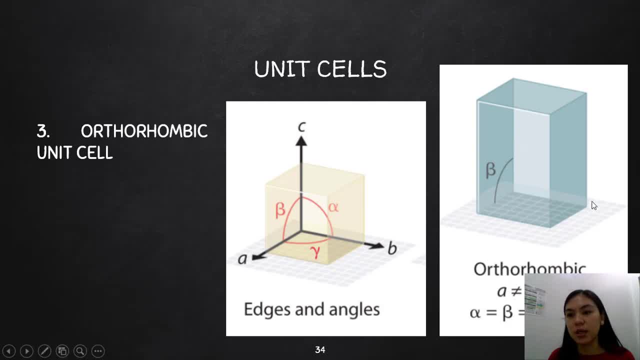 It means that side A is not equal to side B And it is also not equal to side C. So no sides are equal. That's why you have that sign right, The equal sign with a slash. It means not equal, Although all of your angles are equal to each other. 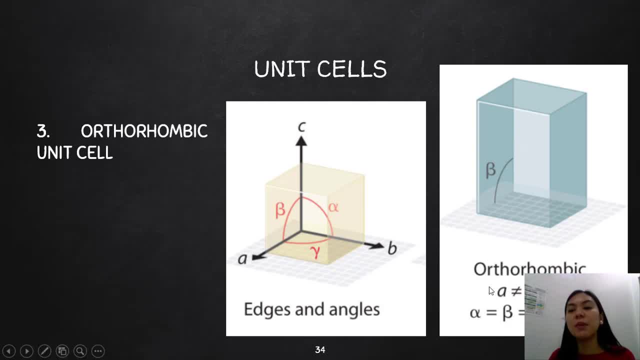 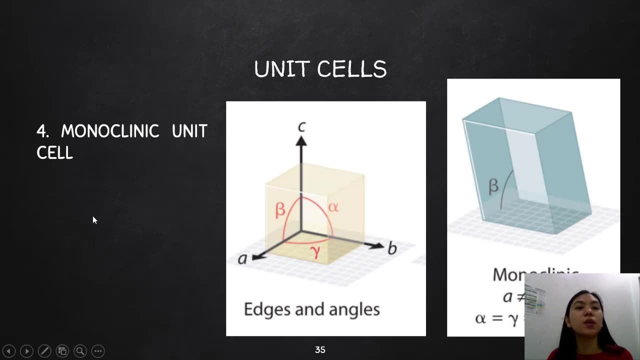 which is 90 degrees. So they are not the same length, although the angles they make with each other is equal to 90 degrees. We call that your orthorhombic unit cell. The fourth one is called your monoclinic unit cell. 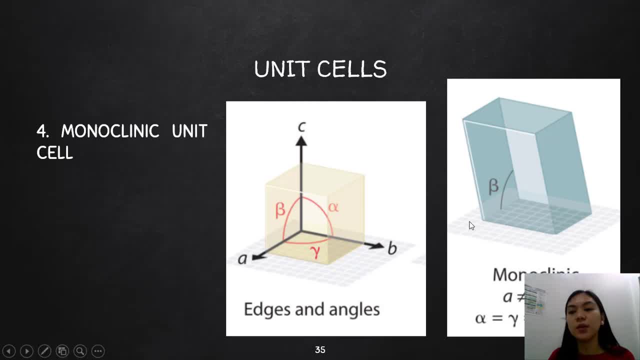 So, as you can see, here the sides are not equal. So your side A is not equal to your side B And they are not both equal. They are also equal to your side C, And a special case here is that, although your angles alpha and gamma is equal to 90 degrees, 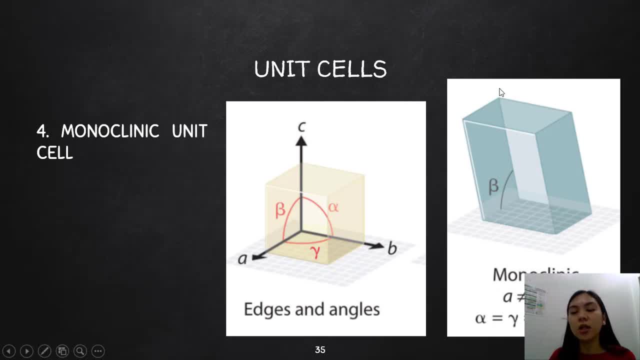 your beta is not equal to 90 degrees. So if you get to see the figure, it is tilted like that because our beta angle is not 90 degrees. So again for your monoclinic, no sides are equal. Your alpha and gamma angle is equal to 90 degrees. 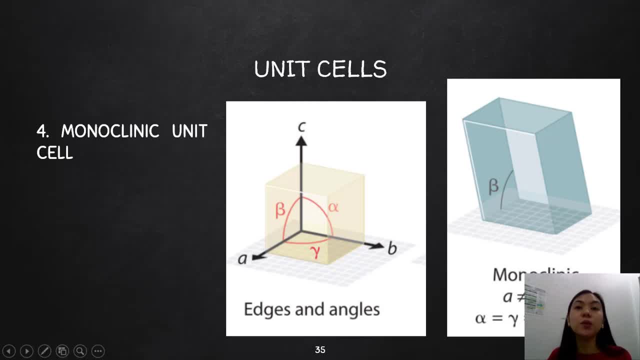 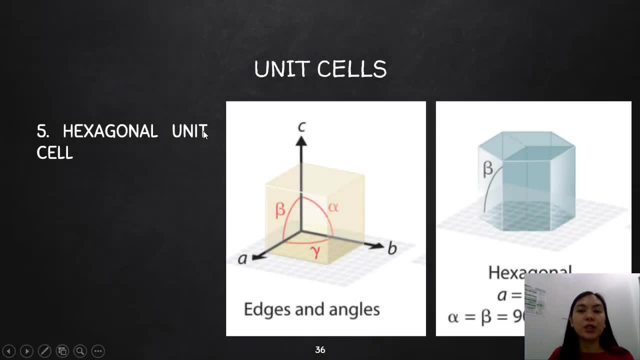 However, your beta angle is not equal to 90 degrees. The fifth type of your unit cell is what we call your hexagonal unit cell. When we say hexagonal unit cell, as represented by this particular figure, your angle A, or rather your side A. 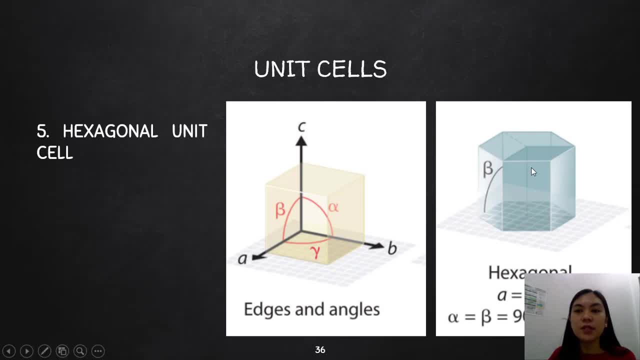 is equal to your side B, So it is like a square. However, your side C is not equal to your side A and B, So in this particular figure, the side C is longer And when we talk about angles, your angles alpha. 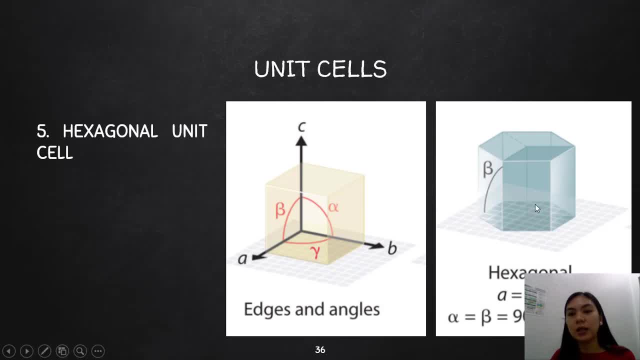 and your angles, beta right, Your angle alpha and beta is equal to 90 degrees. However, your gamma- this one here, your angle gamma, is equal to 120 degrees. Hence the name hexagonal unit cell, Because gamma is 120. 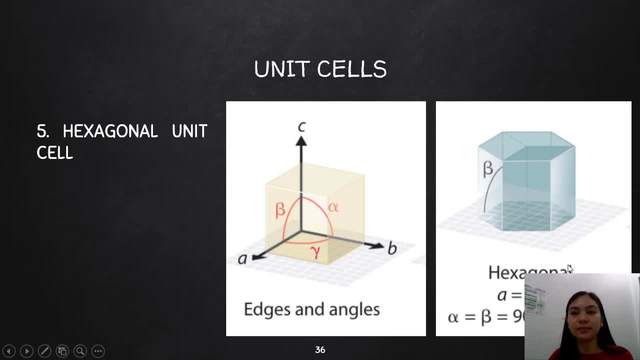 and your alpha beta is 90. So that's the fifth one. Now the sixth type of your unit cell is what we call your rhombohedral unit cell. So when we say rhombohedral unit cell, you can see here from the figure. 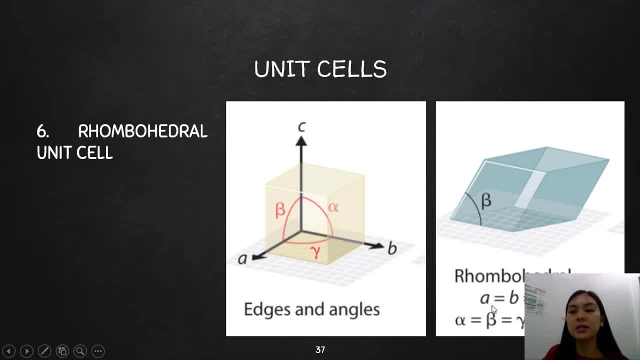 that your angle, that your side A, is actually equal to your side B and it is equal to your side C. Right, It's like a cube. However, the main difference here is that, although your angles alpha, beta and gamma are equal to each other, 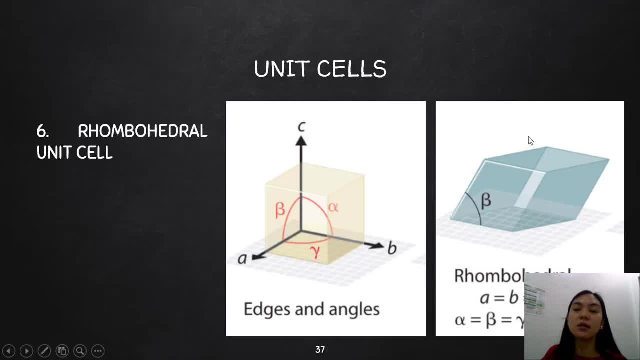 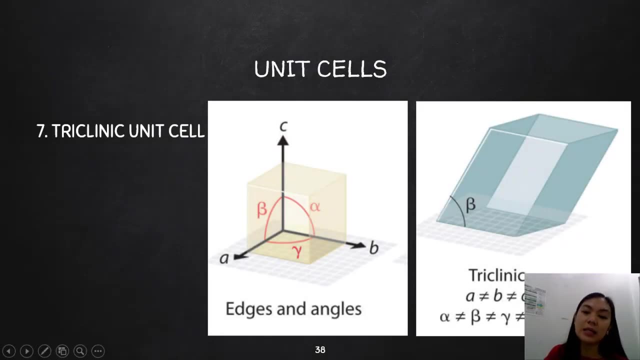 they are not 90 degrees. So, if you can see as a representation of the figure, it's a cube but it's tilted. The angles are tilted because, although they are equal, they are not 90 degrees. And lastly, we have your triclinic unit cell. 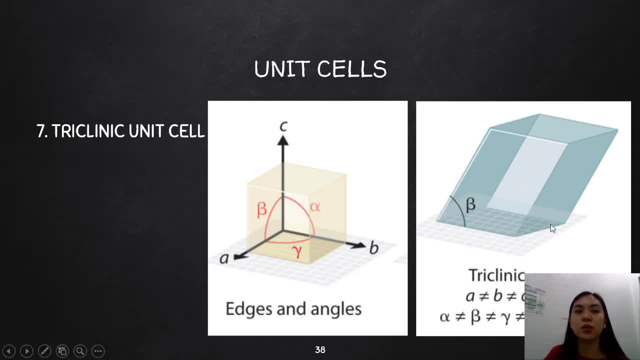 So, as represented by this figure in the right side of your screen you have, your side A is not equal to your side B is also not equal to your side C, and all of the angles are not equal to 90 degrees. So that's all about the triclinic. 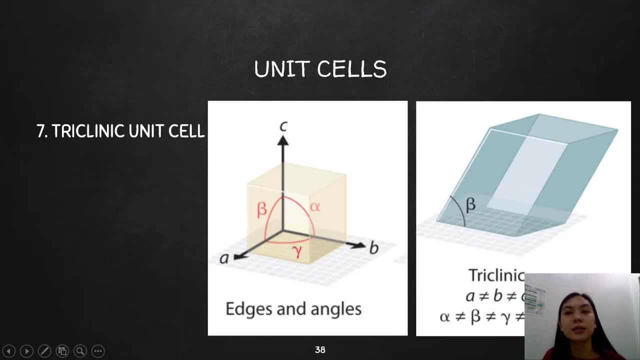 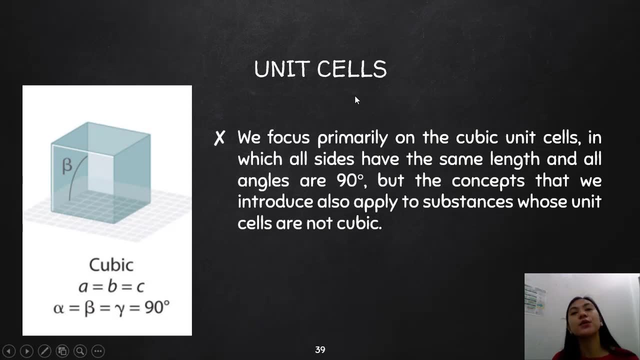 There are no equal edges or angles. Okay, So, of course, among all the seven unit cells that we have been discussing so far, we will focus primarily on your cubic unit cell, in which all sides have the same length and all angles are 90 degrees. 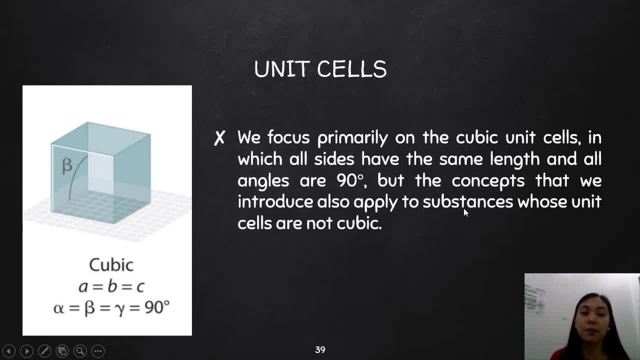 But the concept that we will introduce next. they apply to all the types of unit cells Because, aside from being a cubic unit cell, there are also subtypes. Okay, So, all of the unit cells discussed- you have seven. there are subtypes. 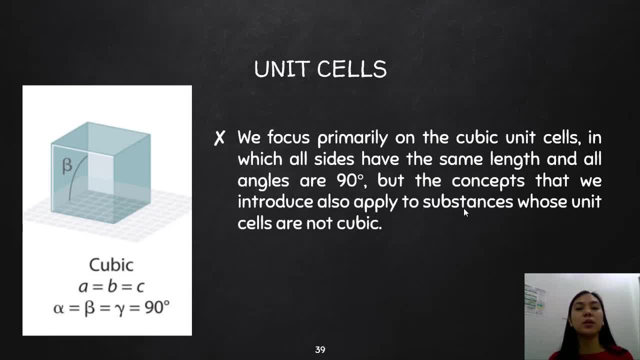 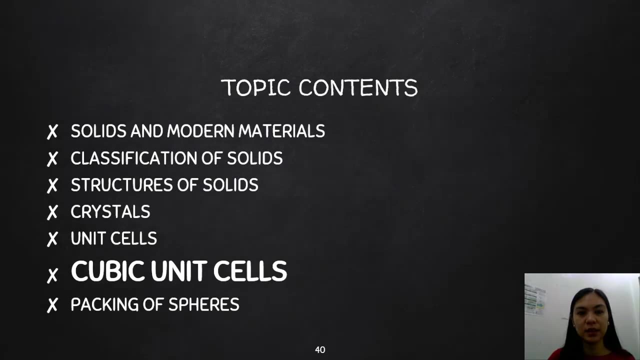 Although the unit cell that we will be talking about, the cubic unit cell, particularly because it is the easiest to understand and the concepts that will be introduced, it also applies to the rest of the unit cells discussed. So you have there, so let's introduce now your cubic unit cells. 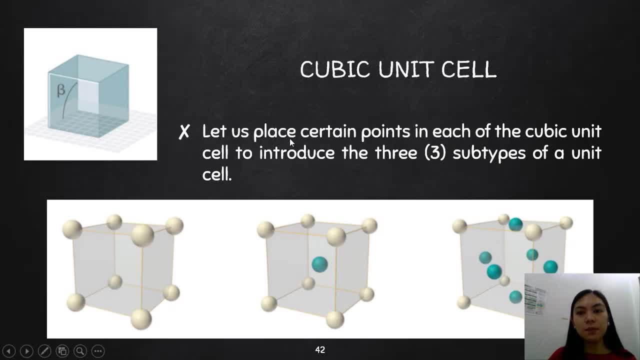 So imagine that this is your cubic unit cell And we place certain points in each of the three unit cells to introduce the three subtypes of the unit cell. So you have here the first one. Imagine we will put. for simplicity, let's imagine that we will place an atom strategically. 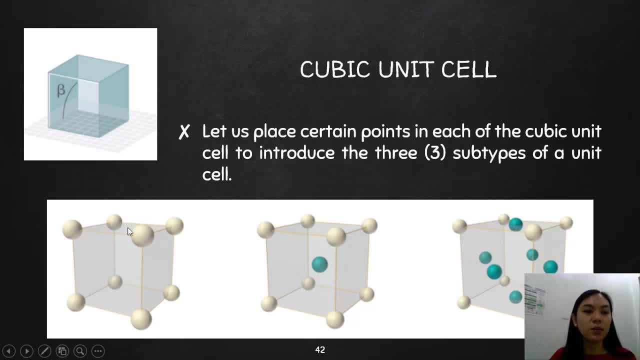 on the edges of that particular unit cell, So it's represented by this particular figure. So this is what you call your cubic unit cell. This is what you call your simple cubic unit cell, Because its atoms are just on the edges of your cube. 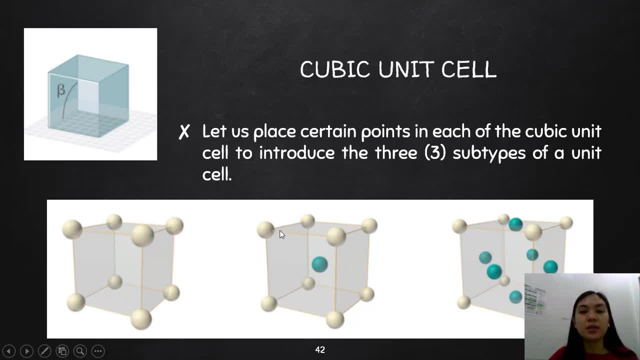 And we also have the second type of your cubic unit cell. So, aside from the eight atoms strategically placed in the corners of the cube, you have another atom in the middle, And the third type is what we call your face-centered cubic unit cell. 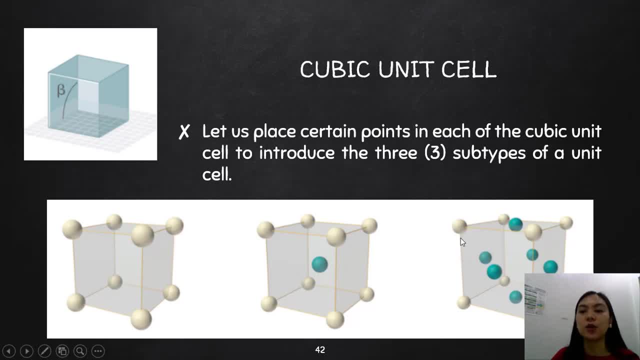 So it's simply parang meron kang eight atoms strategically placed at the corners of the cube, plus an additional atom in each face of the cubic unit, cell Kumbaga. sa bawat side niya meron pang isang atom. 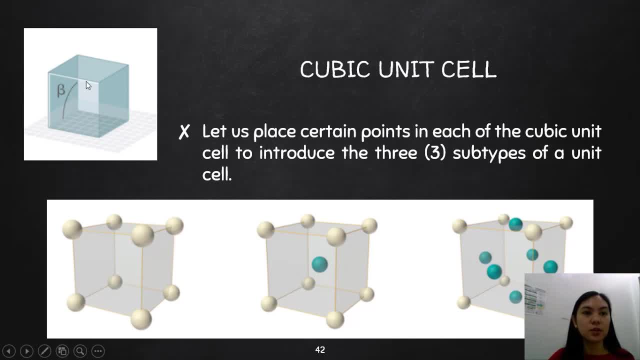 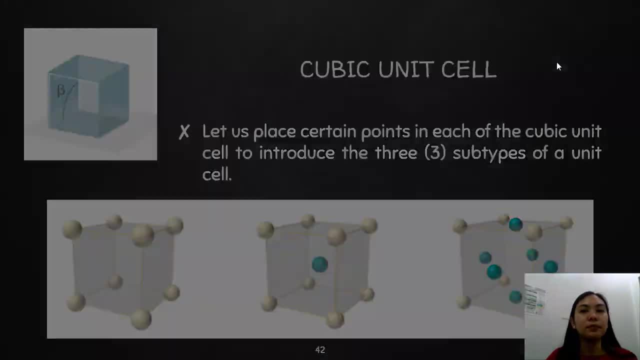 Meron diyan, meron doon, meron doon sa likod, of course, sa baba and sa taas. So that's one. We will take a closer look at each one of them. So your cubic unit cell. 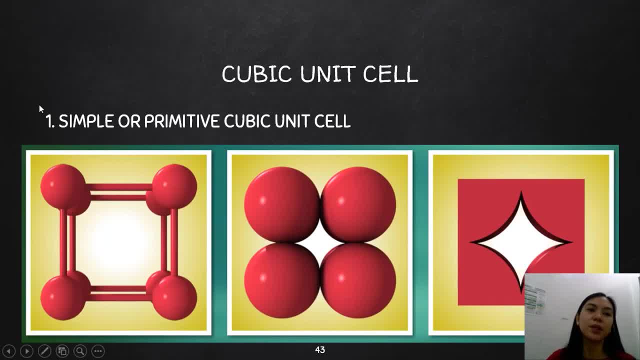 or your. this one is simply called your simple or primitive cubic unit cell. So diba yung figure kanina. as I said, it is strategically placed at each corner of the cube. Diba ganyan siya, Pero. 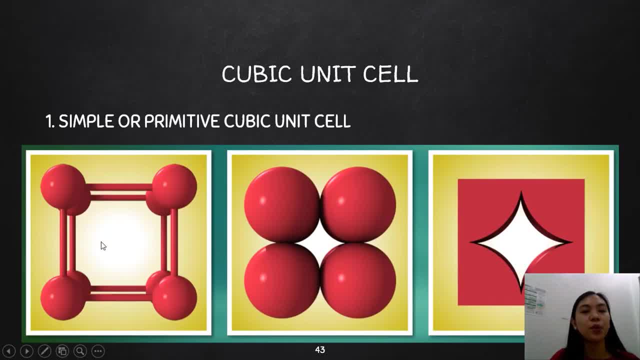 in reality diba, in reality po diba, hindi naman po nag-exist yung distances na yan, Kasi if we represent this particular sphere, this particular sphere as an atom, your atoms are closely packed together. So, in reality, 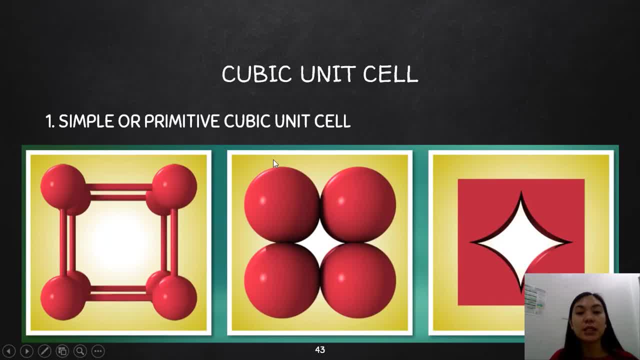 wala naman talaga yung mga rods na yan. It actually looks like this Diba, Parang magkakapatong sila, eh. So it actually looks like this. And your cubic, or your simple primitive cubic cell is this one. 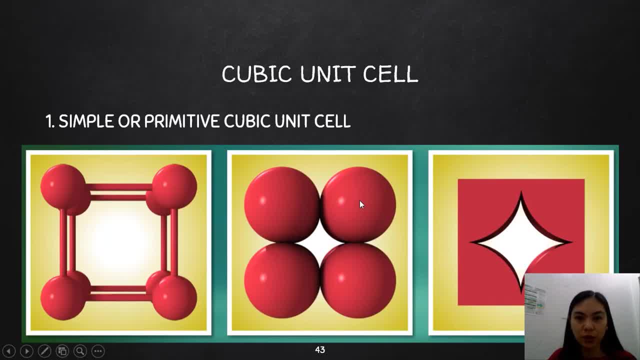 Parang siyang dito siya kinuha, kinot po siya dito sa loob Yan. So pag kinot natin yan, kunyari yung center from center to center, ikakat natin yan. 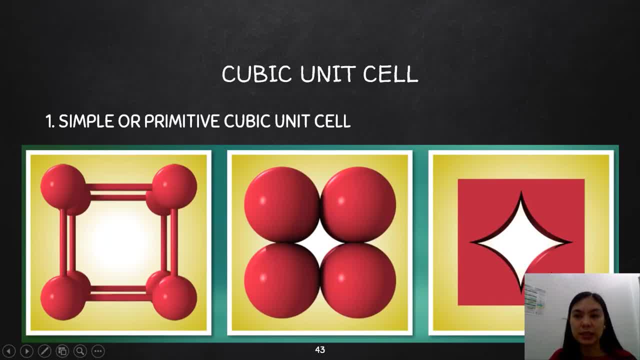 So ganito po yung itsura ng ating cubic unit cell. So, in reality, this is what a unit cell looks like. Okay, Pag we try then to imagine. The next one is what we call your body-centered cubic unit cell. 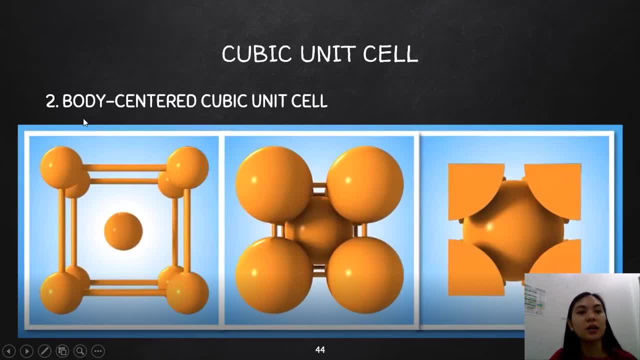 So, diba kanina, in the previous slides that we have, you have eight corner atoms and then you have one atom strategically placed in the center of the cube. So in reality, yung mga atoms, ganito po yung kanyang pagkakapak. 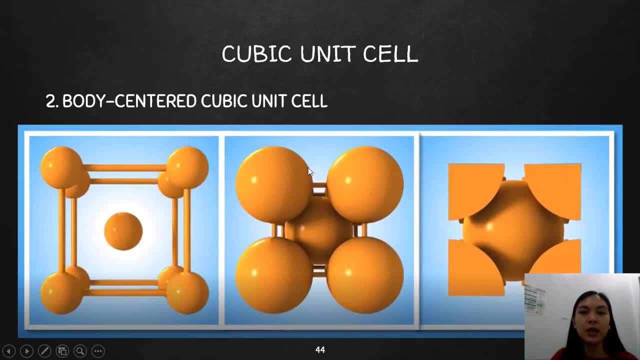 Diba ganyan, So merong isa doon sa gitna. and then of course your eight corner atoms, And if we try to get that particular cubic unit cell, ganito po yung itsura niya. So of course you have one in the center. 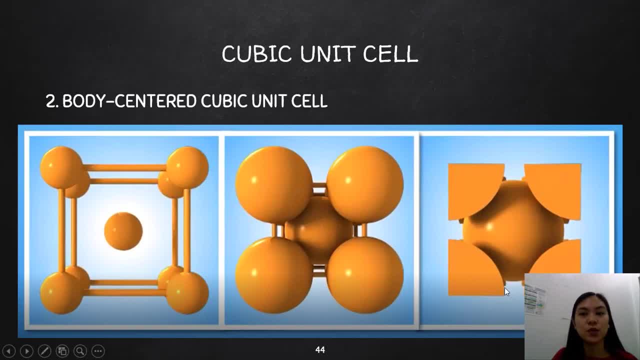 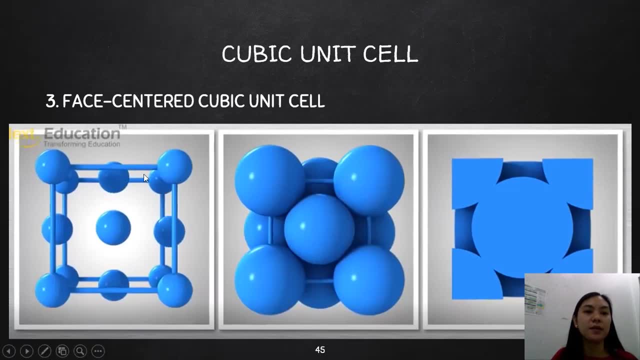 and you have the eight corner Atoms And lastly, your face-centered cubic unit cell. So, as I've stated earlier, aside from the eight corner atoms, meron ka in each face of the cube. So meron sa taas. 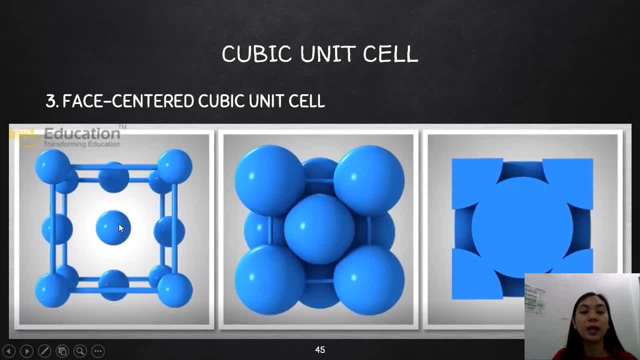 sa baba, sa right, sa left and, of course, sa front and back, Such that, if we take a closer look at how it actually looks, like diba, Wala naman po talaga yung mga atoms. Wala naman po talaga yung mga atoms na yan. 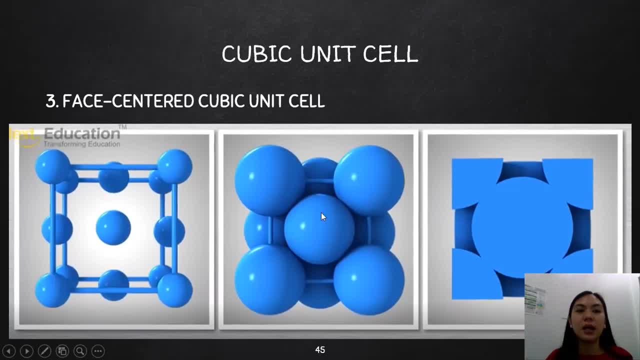 Ganito yung itsura niya, Para siyang na-compress Ganyan. And if we try to get the cubic unit cell or the unit cell in this particular shape, ganito po yung kanyang magiging itsura. 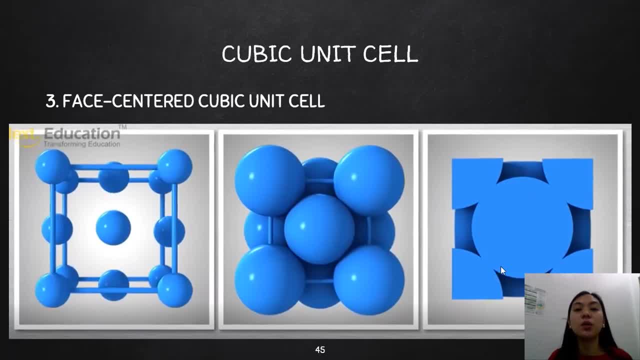 That's how a face-centered cubic cell, cubic unit cell, looks like Diba. So, as I said, cubic unit cell yung pinag-uusapan natin, Pero all of this simple body-centered and face-centered unit cell. 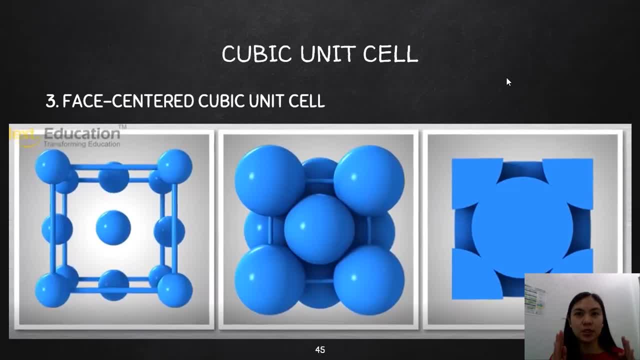 is applicable to all types of unit cell. Mas, madali lang po kasi siyang ma-imagine when we talk about a cube, Kasi it's the simplest shape that we have among all of the unit cells that are presented. So it says here: 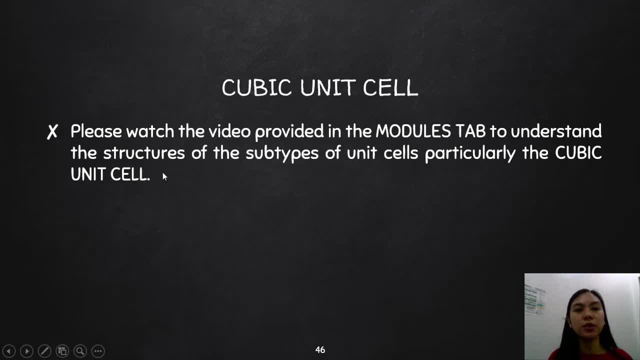 please watch the video provided in the modules tab to understand the structures of the subtypes of unit cells, particularly the cubic unit cell. I will be posting a video in your modules tab in Canvas, para po mas ma-imagine nyo siya how it actually looks like. 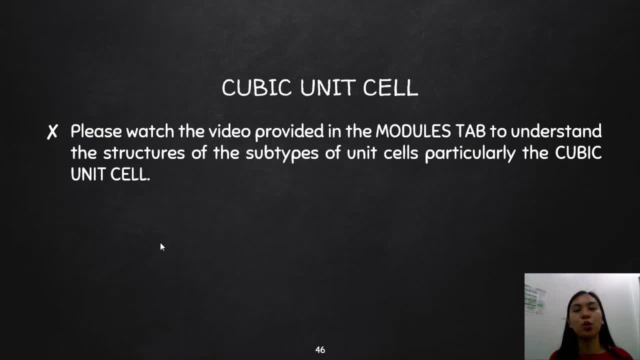 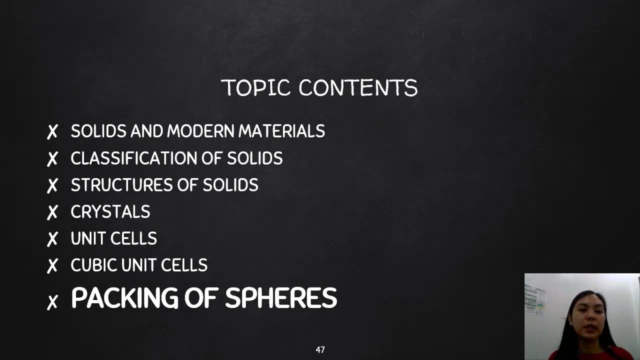 Kasi medyo doon gumagalaw-galaw yung image, So it's better na makita nyo siya visually, yung paggalaw-galaw, para you get to understand these subtypes better. Okay, Now let's go to the last part. 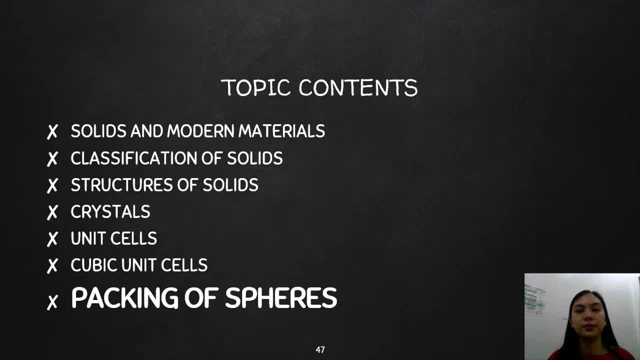 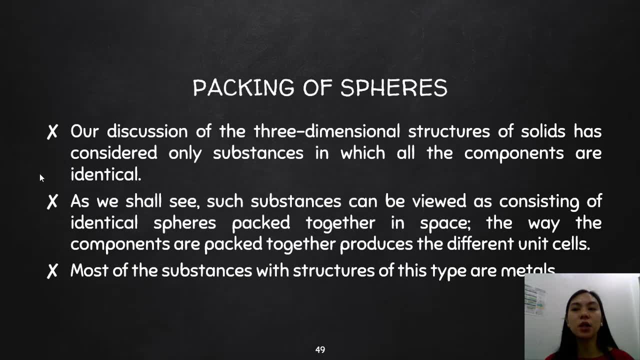 We call this the packing of spheres. So it says here. our discussion of the three-dimensional structures of solid has considered only substances in which all of the components are identical. As we shall see, such substances can be viewed as consisting of identical spheres packed together in space. 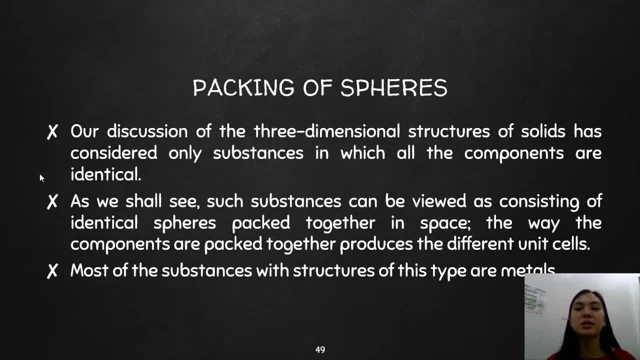 The way the components are packed together produces the different unit cells. Most of the substances, substances with structures of these types, are metals. So ang sinasabi lang po natin di ba: siyempre, if you have an atom, 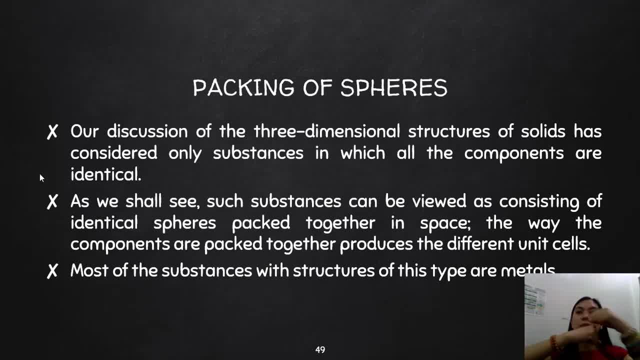 di ba, pag nakita nyo naman po doon sa mga unit cells di ba, they are closely packed together, Parang they are stacked, parang kumbaga mayroon siyang atom sa left sa right. so di ba nakompress siya. 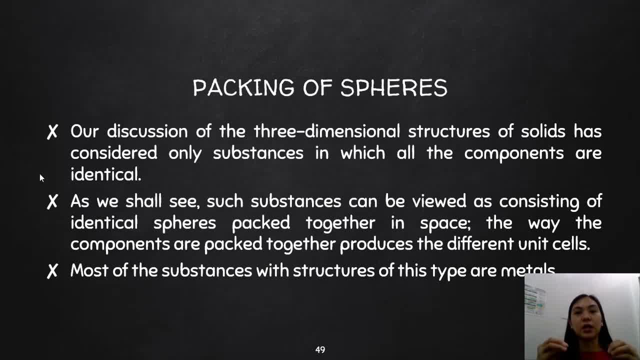 Pero paano po ba nagpapatong-patong yung mga atoms na iyon? That is what we will be talking about in this type, in this particular topic, where we are packing off spheres. So it says here: simple cubic structure. 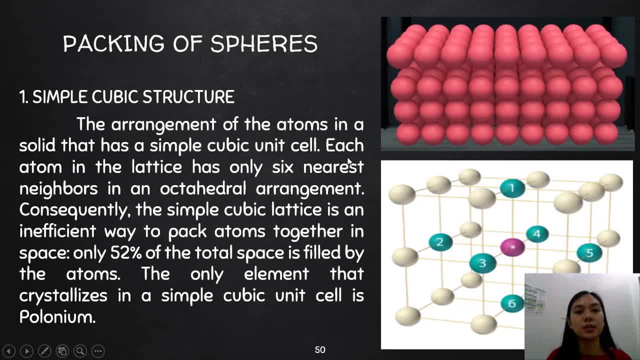 The arrangement of the atoms in the solid that has a simple cubic unit cell. Each atom in the lattice has only six nearest neighbors in an octahedral arrangement. Consequently, the simple cubic lattice is an inefficient way to pack atoms together in space, since only 52% of the total space 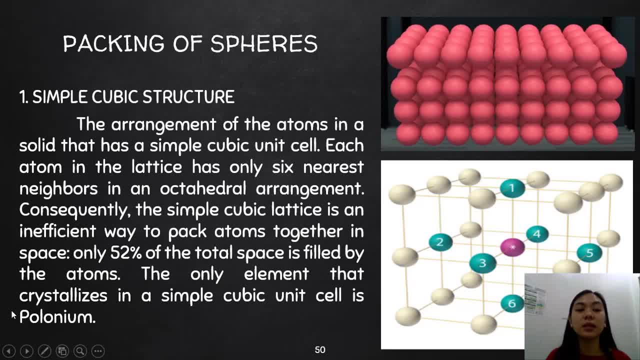 is filled by the atoms. The only element that is that crystallizes in a simple cubic cell is your element, polonium. So very rare po yung magkakaroon tayo ng simple cubic unit cell, kasi it's not very efficient in terms of packing. 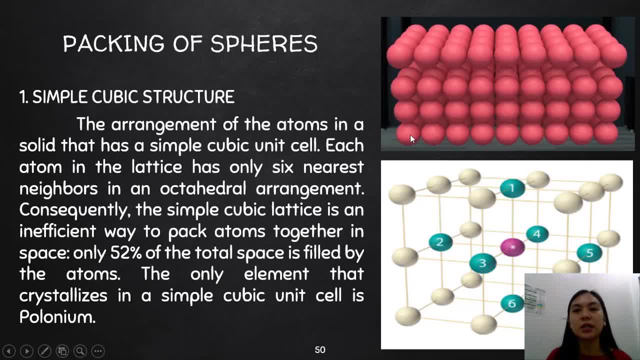 It's only your element, polonium Di ba. so parang ganito: example mo, yung isang sphere, dyan, is an atom Di ba, para lang siyang nag-stack up on top of each other. So ito pareho lang lang. 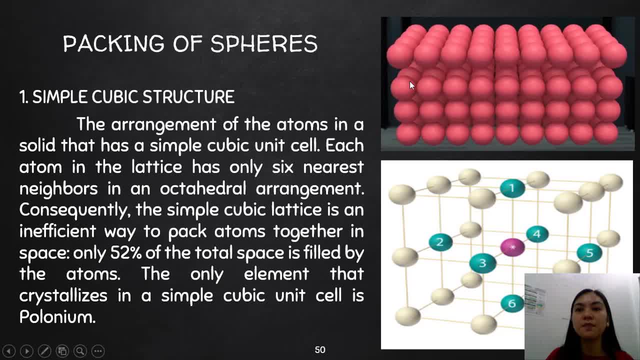 pagkaka-pack dito or pagkaka-stack and ganyan ganyan. So pareho lang po kung paano-paano sila nagpatong Such that if you take a look di ba ayan o. 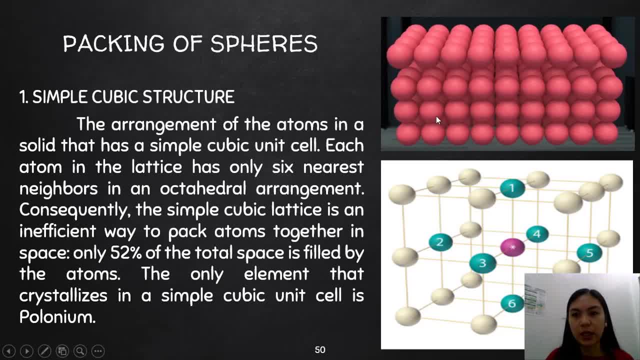 yan po yung inyong cubic unit cell. If we take a look at that And pagpunta ka dun sa may bandang gitna. so imagine mo, this is the atom na nasa gitna, Di ba? parang ilang atoms ba yung naka-attach sa kanya? 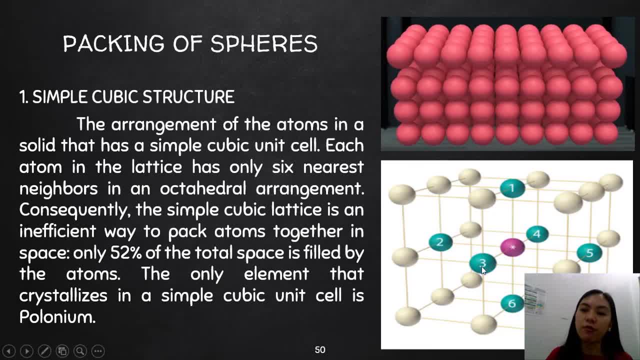 Of course you have the atom on the back, on the front, and then you have the atom number 5 sa left, sa right side niya. the atom number 2 on the right, or rather left side, left side of this atom is atom number 2,. 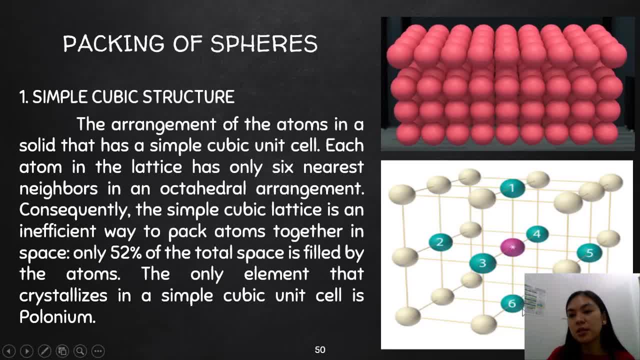 sa right side is 5, sa taas is 1, sa baba is 6.. So kumbaga sa isang particular atom, may 6 po na atoms na naka-attach. Yan po yung simple cubic structure. 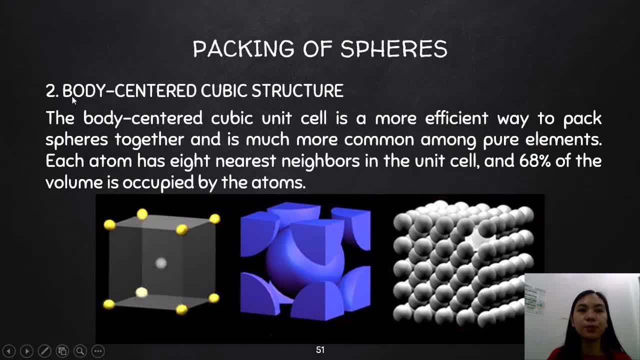 Now let's take a look at the other type. So you have your body-centered cubic structure. So the body-centered cubic unit cell is a more efficient way to pack spheres together and is much more commonly among pure elements. Each atom has 8 nearest neighbors. 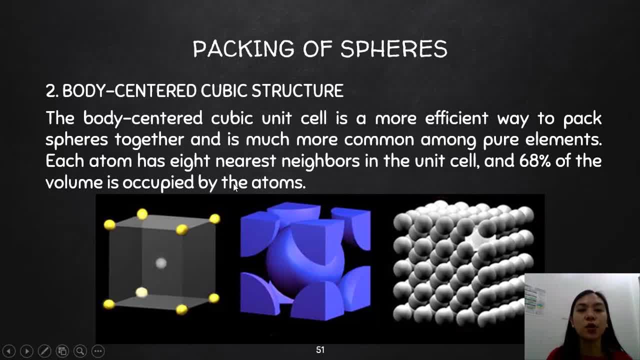 in the unit cell and 68% of the volume is occupied by the atom. So, kumbaga, di ba ito nakita na natin? ganyan yung itsura niya. But when a BCC is stuck together, ganito yung itsura niya. 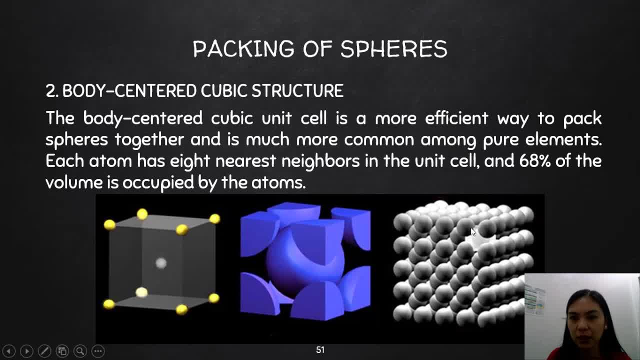 Imagine nyo yun yung center, Tapos may naka-attach na, of course, 1,, 2,, 3,, 4,, 5,, 6,, 7, 8.. Nandun sa likod. 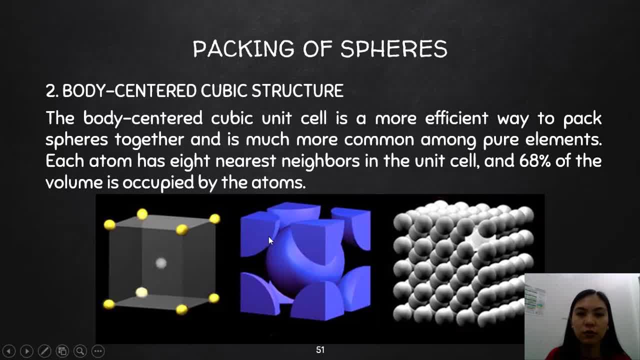 Parang ganito siya: 1,, 2,, 3,, 4,, 5,, 6,, 7,, 8.. So sa isang atom na nasa gitna, merong 8 atoms na naka-attach sa kanya. 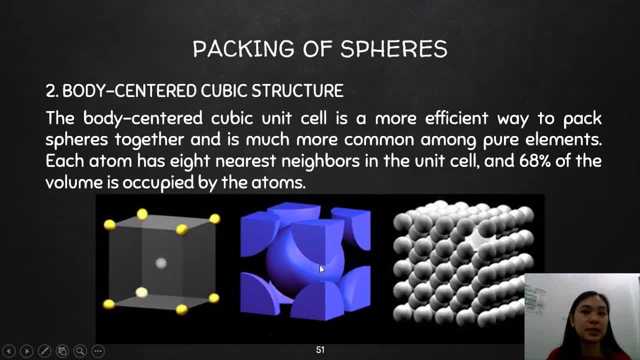 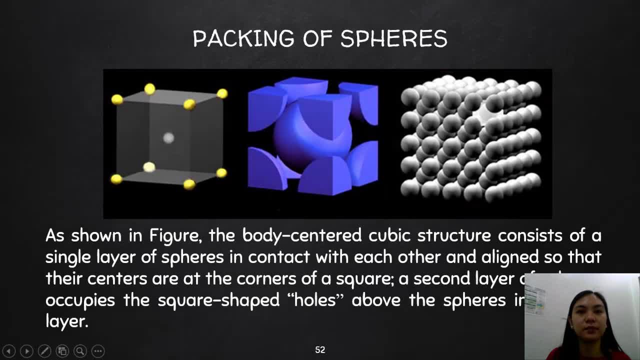 And the volume sa loob is around 68%, So mas efficient siya in terms of sa pagkakapak ng mga atoms. Sinasabi lang po dito yung diniscuss ko na kanina, Di ba Kunyari merong kang apat sa baba. 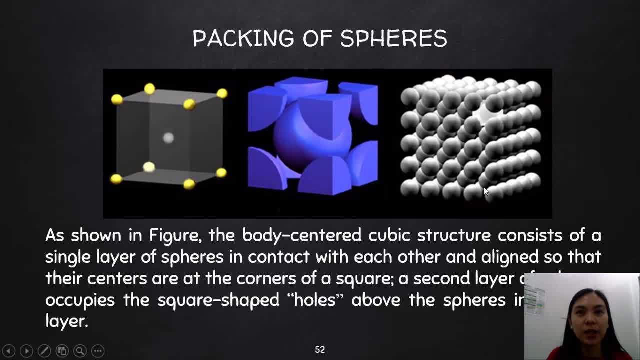 parang yung susunod na layer is ilalagay doon sa parang gitna nung square na yun. Kung we imagine that these spheres are your atoms, So ganun lang siya nagpatumpal. That's how you do the BCC. 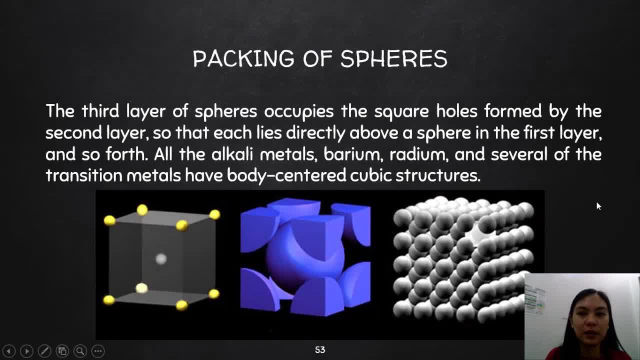 structure. The third layer of the spheres occupies the square formed by the second layer, so that each lies directly above the sphere in the first layer. Kung ano po yung. kung baga, if this is your first layer, tapos yun yung. 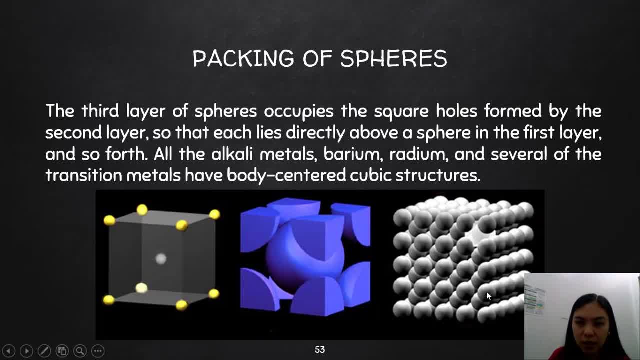 second layer mo, yung third layer mo, parang the same lang siya ng pagkaka-stack doon sa first layer mo, Di ba? So yung kung baga dito sa structure na to your first layer is packed the same as your third layer. 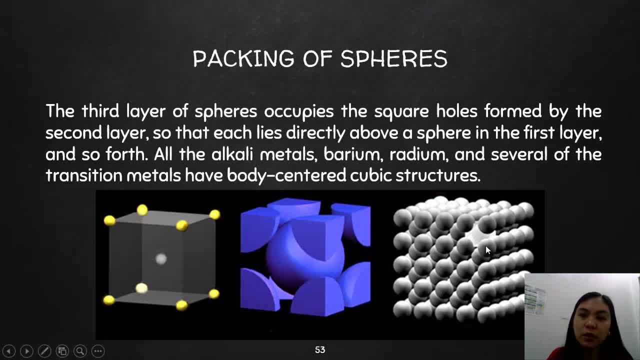 and the same as your fifth layer and the same as your seventh layer and the same as your ninth layer, Tapos yung second, fourth, sixth and eighth layer, pareho sila ng pagkaka-pack. It says here: 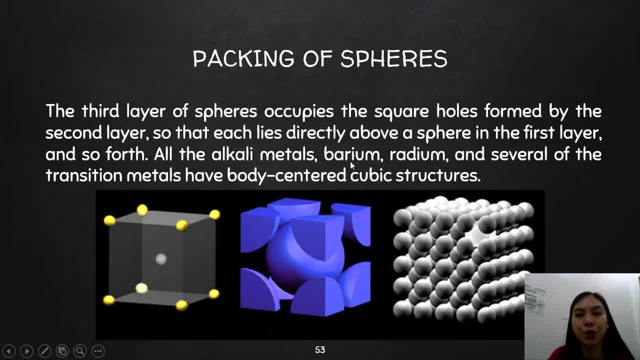 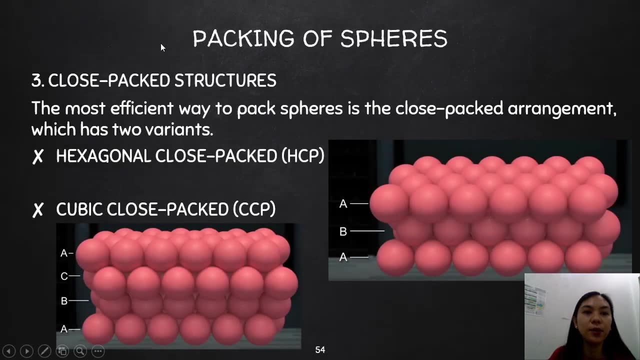 all the alkali metals, such as your barium radium and several of the transition metals have a BCC structure. So yan lang po yung example ng mga solids which follows this particular type of packing And the third type of your spheres. 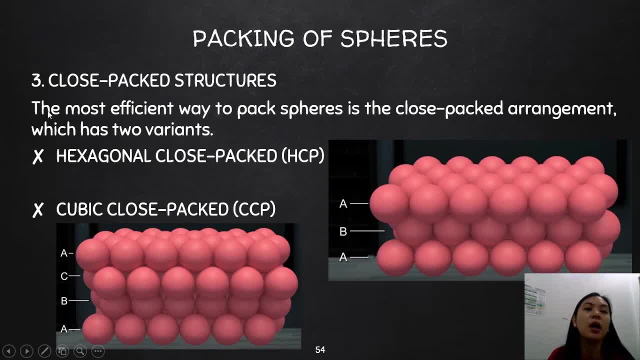 packing is called your closed pack structures. Among the three, this is the most efficient way to pack spheres, kasi mas malaki yung volume na na-occupy ng atoms. So you have two variants for this type of packing. You have your hexagonal closed pack. 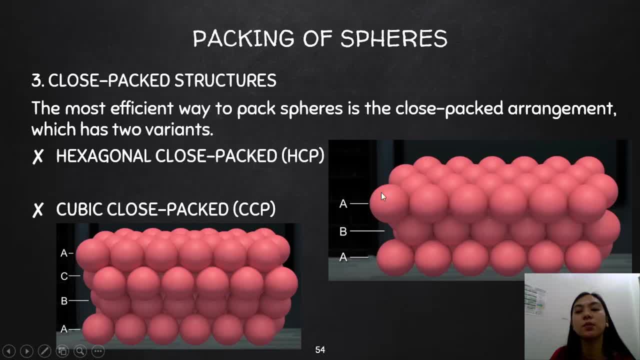 or we commonly denote it as your HCP. So makikita mo dito ganyan siya And your cubic closed pack, or what we commonly know as your CCP, ganito naman siya. So kung baga si letter A. 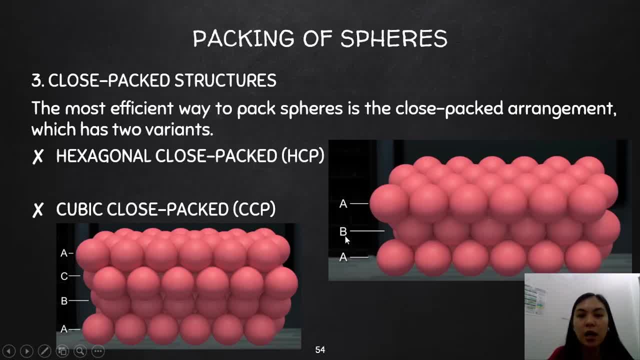 or si first layer is pareho kay third layer. However, iba dun sa BCC yung second layer mo, kasi nakalagay siya dun sa gitna ng square e ito nakalagay siya dun sa depression, what we call. 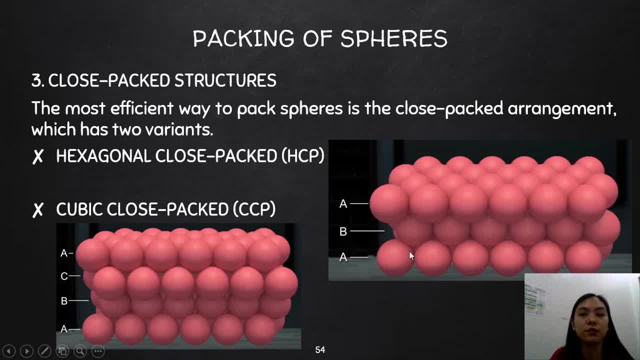 your depression or space in between the two atoms on the first layer. Tapos naman, ito naman iba po yung third layer. kung paano kasi naipatong si third layer For you to understand it better? 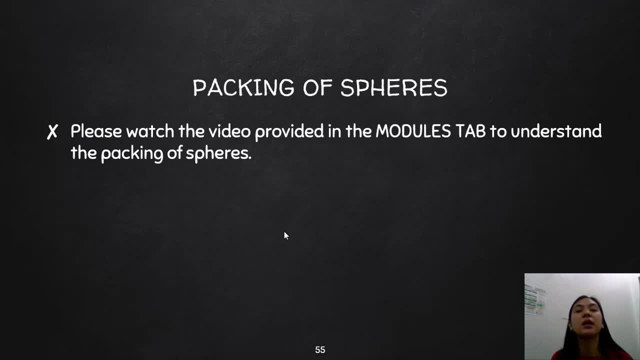 how this particular spheres are packed. another video is provided to you in the modules tab. Mas maganda ito kasi mas natag dito. At least ngayon, you have already an idea, and the video will just supplement the idea that you already have. 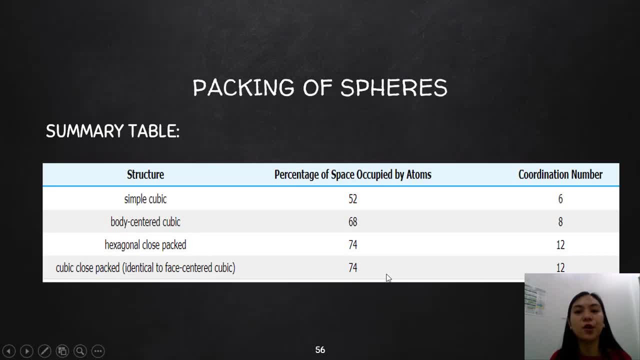 So if we have a summary table, percentage of space occupied by atom, you have this: For simple cubic, 52% of the volume is occupied. for a BCC or your body centered, it's 68%. Your hexagonal, your HCP. 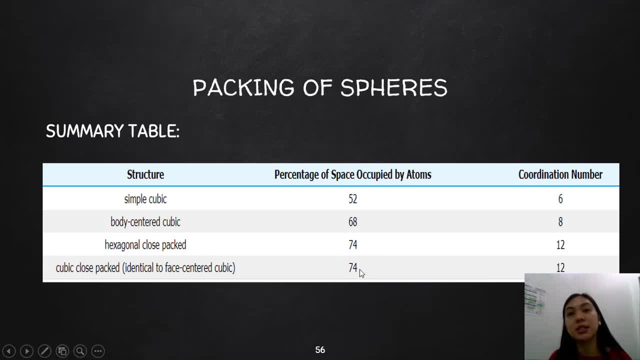 and your CCP occupy 74% of the total volume, So mas preferred ito, kasi ito na po yung mga mas matitibay na solids, And when we talk about your coordination number as indicated here, kumbaga ito yung number. 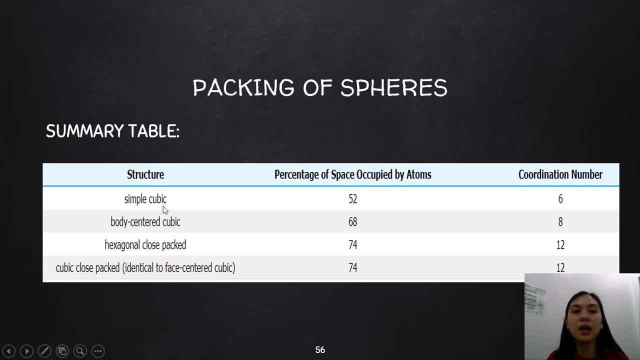 of atoms na nakadikit sa kanya. Diba parang sa simple cubic kanina, kung may atom kasagitna yung neighboring atoms niya, ilan po ba yung neighboring atoms niya na nakadikit sa kanya? 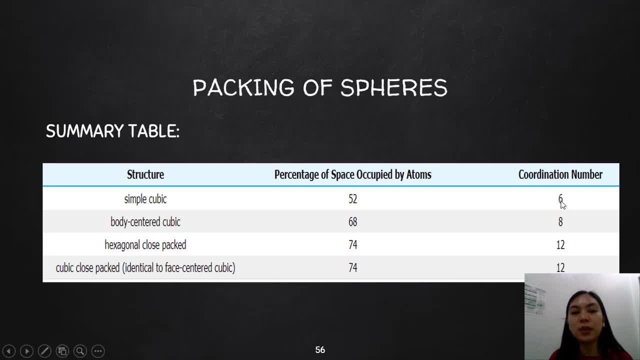 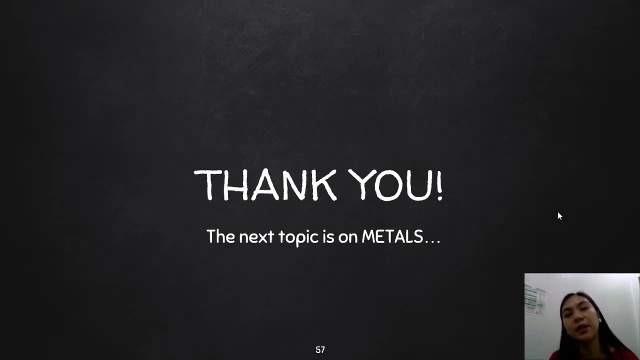 That's actually your coordination number. So for your simple cubic, it's 6.. For your BCC, it's 8.. For your HCP and your CCP it's actually 12.. So thank you for listening class. We will be having the next topic.